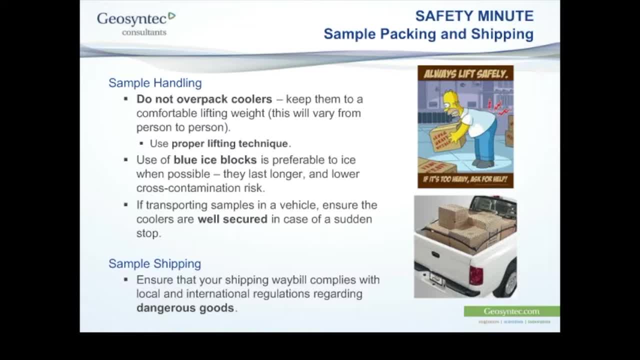 So for the safety minute topic today, I've selected sample packing and shipping, and this is probably the aspect of treatability studies that our clients are coming most in direct contact with- that is, actually getting us the sample material in order to conduct these studies. So, from a safety perspective, one of the key issues with sample handling- 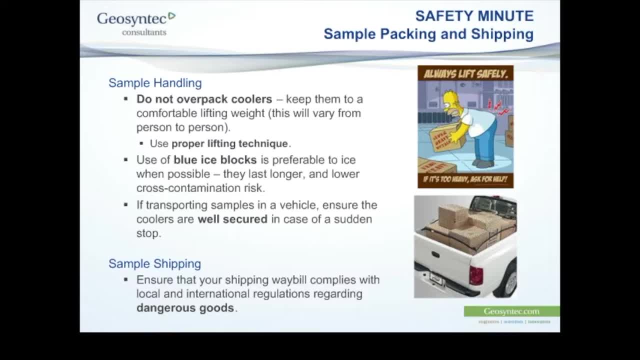 is the manual handling of Eskies filled with samples and ice or cooler blocks. As many of us know, these things get really heavy really fast. It doesn't take that many samples for your Eskie to become very guilty, and this is not rocket science, but just fill. 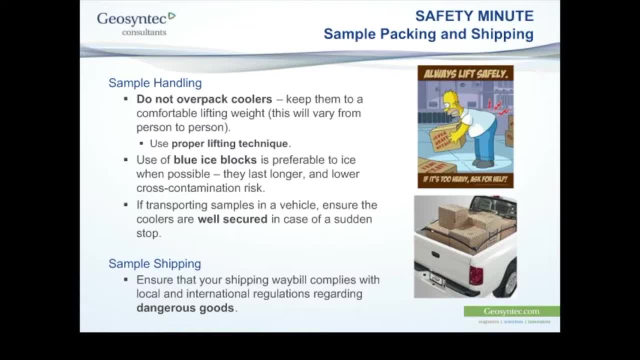 your coolers to the weight that you are comfortable lifting. Maybe plan on having extra coolers and try to shove everything into the smallest number of coolers. You'll save your back and you'll avoid injury doing it this way. and, of course, always use proper lifting technique. 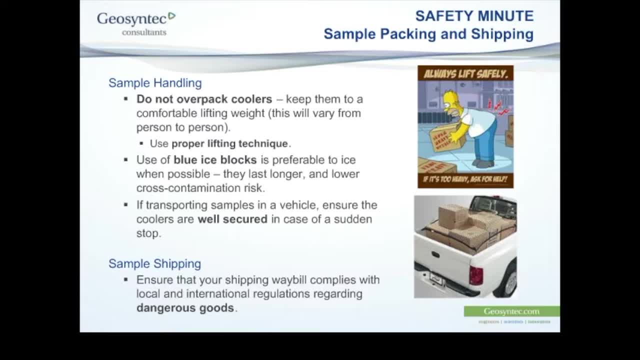 when lifting heavy coolers. This is probably more of a quality issue than a safety issue, but we strongly recommend using blue ice blocks rather than wet ice for keeping samples cool. The main reason for this is that when ice melts, it will melt the sample, and that's. 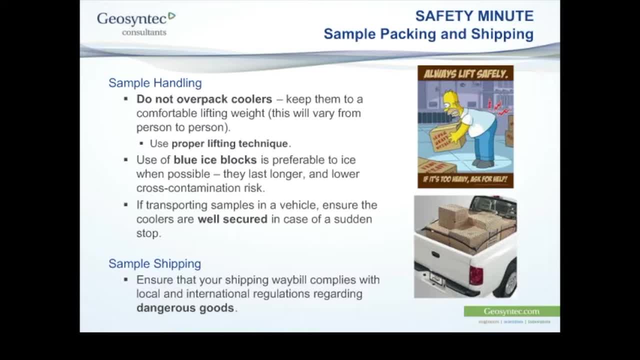 the main reason for this. So we've got a lot of different ways of doing this and we're going to talk a little bit more about that in just a few minutes. Your samples are floating around in melt water. The potential for cross-contamination is. 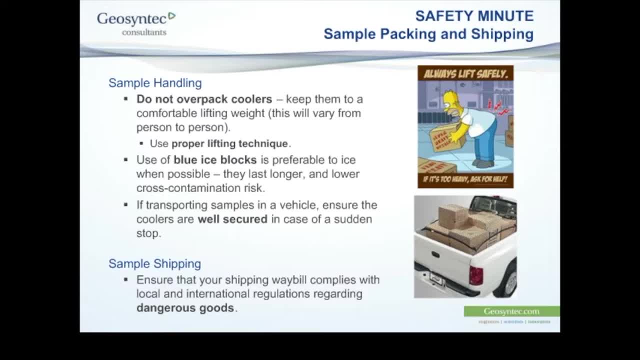 much greater. It can be a safety risk if there is transfer of contaminants into that melt water and, for example, you get a leak from your cooler during transport. So we strongly recommend using blue ice blocks rather than wet ice, and this just takes a little bit. 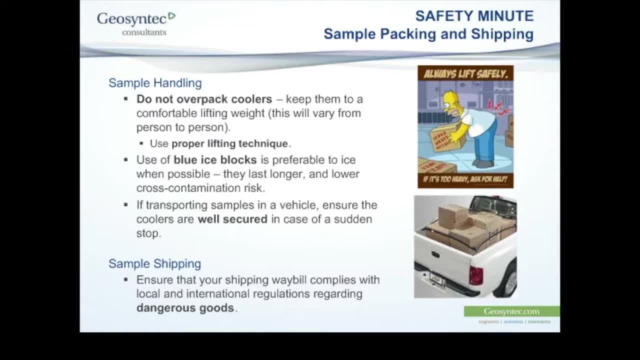 of advanced preparation, because you can often go to your local market and buy frozen blue ice blocks. You just have to have them on hand the night before. If you're transporting your samples yourself- if you're not getting them picked up from site by a courier- just make sure that your coolers are well secured. Often coolers have 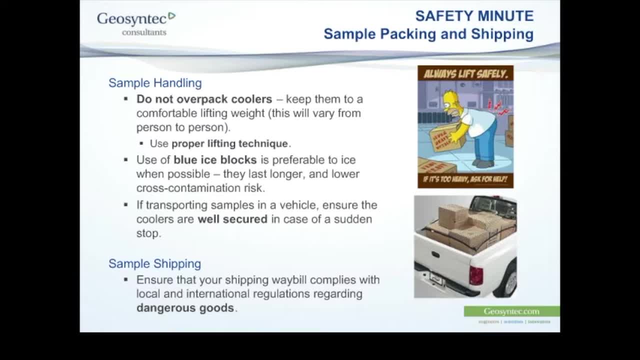 a hard plastic shell. They're going to slip and move around very easily if you have to slow down quickly, if you get rear-ended, if you're in an accident, and a heavy cooler moving at high speed in your vehicle is a good idea. 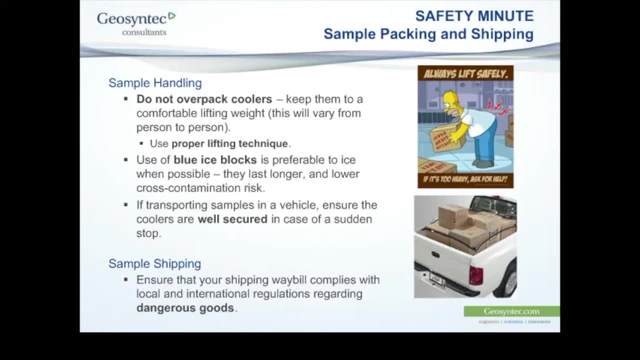 It's an extremely dangerous thing to happen. On the lighter side, you may break your sample containers. On the worse side, you can have a devastating injury from this sort of thing. And finally, with shipping your samples, just ensure that on your shipping waybill your 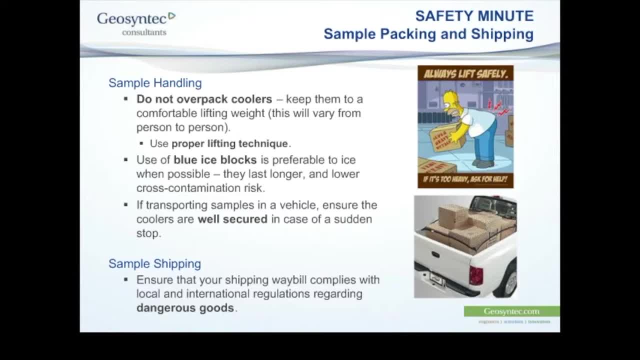 sample shipment complies with any local or international regulations regarding dangerous goods. Now Sandra will touch on in this presentation the shipping of environmental samples to Serum Lab. It does not constitute the shipment of dangerous goods. We do have detailed guidance in that regard that we provide to our clients. 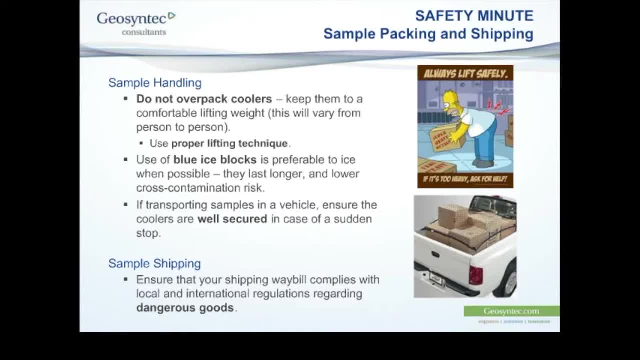 when they're shipping samples. It is not a dangerous good shipping situation when you're shipping environmental samples to us. But as a general precaution, if you're ever shipping around samples locally or internationally, just check first that you're shipping the samples locally. And if you're ever shipping the samples locally, just make sure that you're. in compliance. So, moving right along, Chio Syntec Consultants. who are we? Well, we're an environmental consultancy that was founded in the United States just over 30 years ago. We have a bit over 1,000 employees based in a bit over 60 offices. Our primary base is in the United. 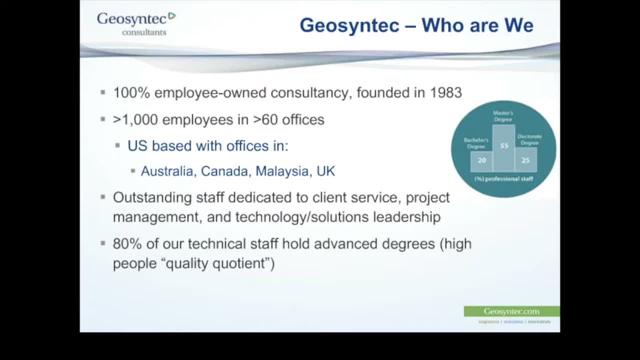 States, but we have local presence in Australia, Canada, Malaysia, the United Kingdom and we service a lot of markets beyond those from those hubs. As an overarching view of Chio Syntec Consultants, we really focus on targeting the difficult work, the challenging work. 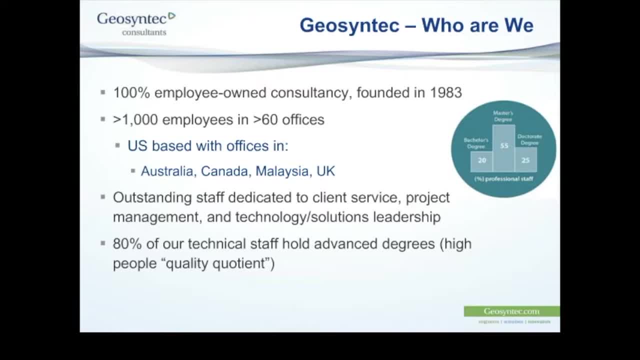 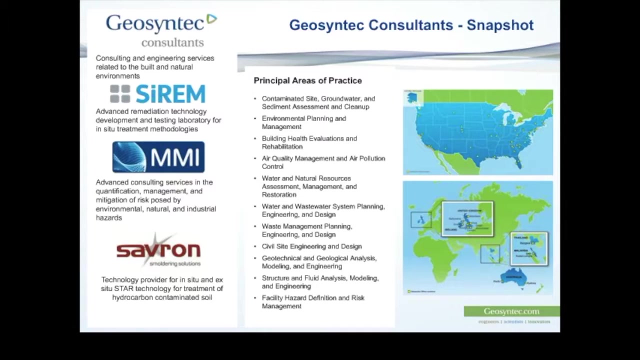 the projects that others may not be equipped to deliver or provide advice on. And we do that by really targeting staff with excellent academic credentials, excellent industry experience, and facilitating that to provide advice that others may not be able to provide. in our field, Chio Syntec Consultants is a family of companies. Some of those include Serum. That will be. 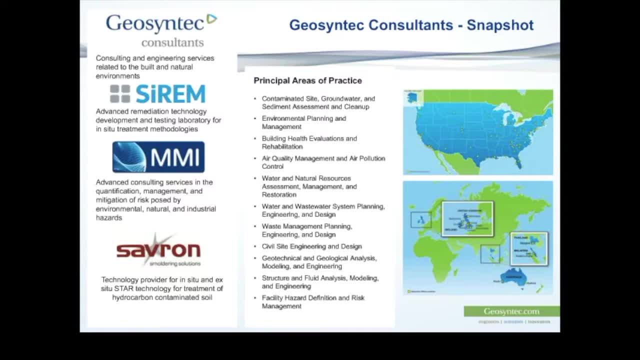 the topic of today's discussion. Sandra will cover Serum's capabilities in great detail, so I won't address those now. Chio Syntec Engineering, which is a safety and risk engineering consultancy, focuses on the quantification and management of risk posed by natural hazards and industrial process. 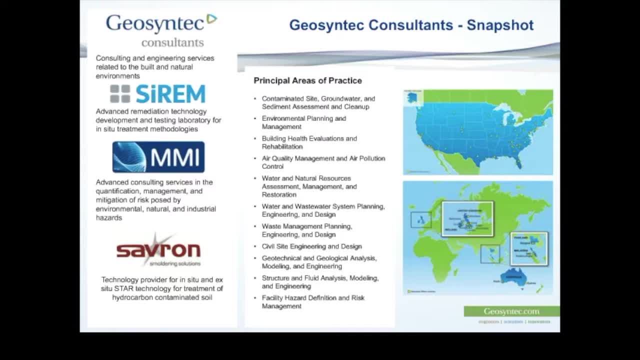 hazards Savron, which is a company that licenses a remediation technology developed by Chio Syntec, which is the STAR technology, which is based on smoldering combustion of bean apples. It's quite an interesting technology. Chio Syntec Engineering, which is a company that licenses a remediation technology, developed. 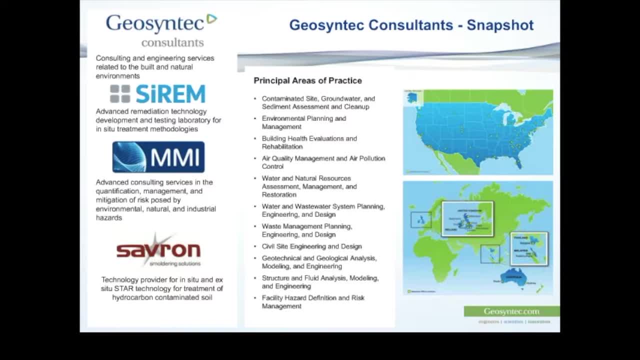 by Chio Syntec, which is based on smoldering combustion of bean apples. It's quite an interesting technology and will definitely be one of our upcoming topics. There is one I haven't listed here, which is our newest member, OptiRTC. I will hold 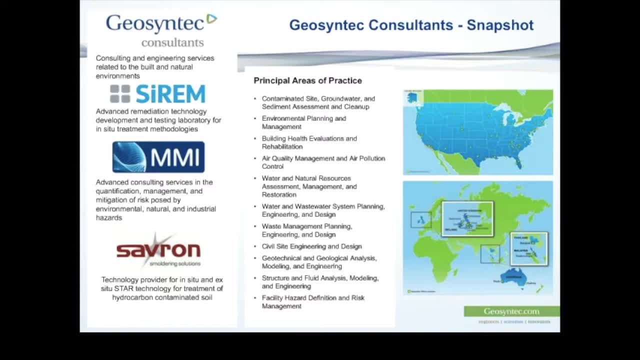 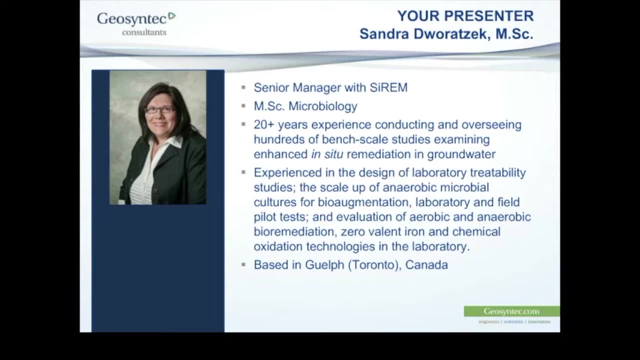 on giving details on that one until I've actually got it up on the slide. but newest member of the Chio Syntec family. On to our presenter. today, Our presenter is Sandra Dwortvik, who is the senior manager with Serum. Suffice to say that Sandra has lots and lots of experience. She's been working. 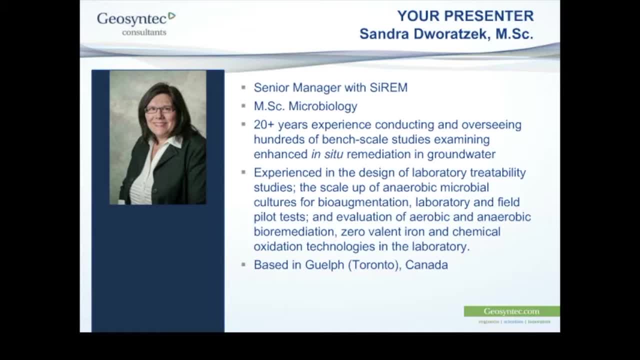 with the design and the implementation and the interpretation of laboratory studies to evaluate remediation techniques for soil groundwater sediment across a broad range of remediation types and techniques. I will let Sandra take it from there, as that is the topic of our discussion today. Sandra, thank you very much for your time and for 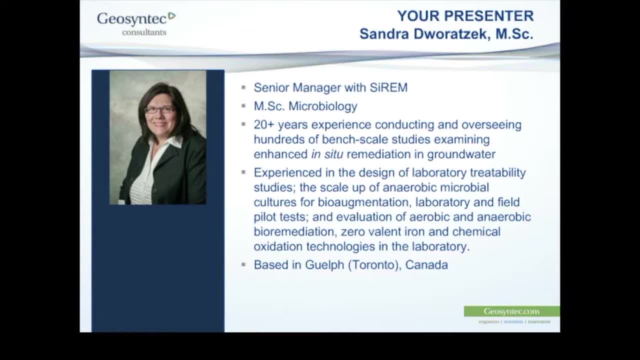 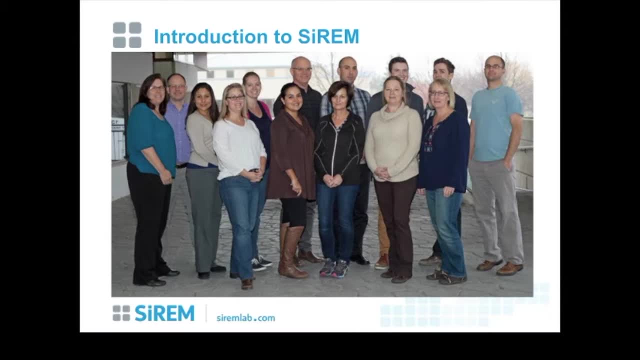 as always, accommodating our time zone differences. Thank you, Without further ado, over to Sandra. Thank you very much. Good evening everyone. I'd like to introduce you to Serum. My name is Sandra Dwortvik and I'm on the photograph on the slide here. I'm on the very left-hand. 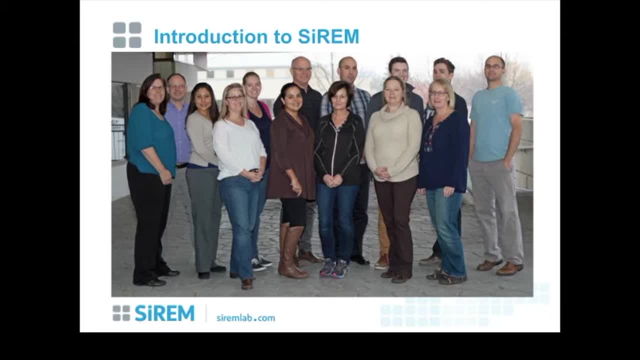 side. here I am one of three senior managers at Serum. I work with Phil Dennis, who's right next to me in the picture, and Jeff Roberts, here over in the middle of the picture. We all report to our director, Peter Dollar. 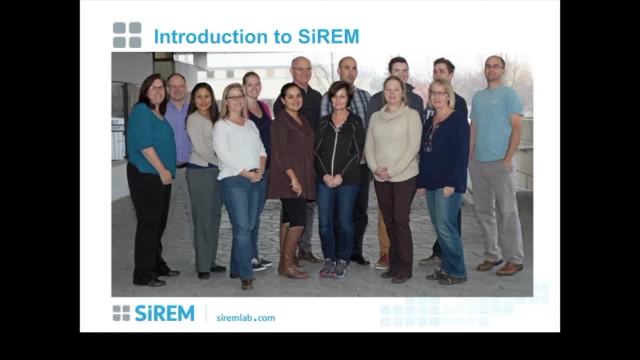 He was a hydrogeologist. Jeff Phil and I are all environmental scientists, microbiologists, molecular biologists, and we manage this group of laboratory technicians who are chemists, microbiologists, molecular biologists, biotechnology technicians, that sort of people in the laboratory. 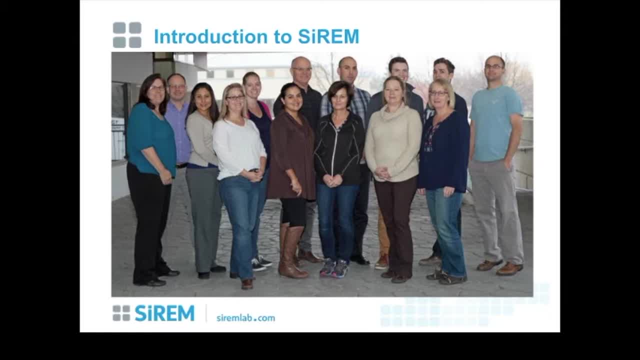 at Serum. Serum has been around since 2002, and we provide laboratory testing services and products for remediation not only of groundwater but of soil. How are you going to help us? Do you have any recommendations for us on how to aid our 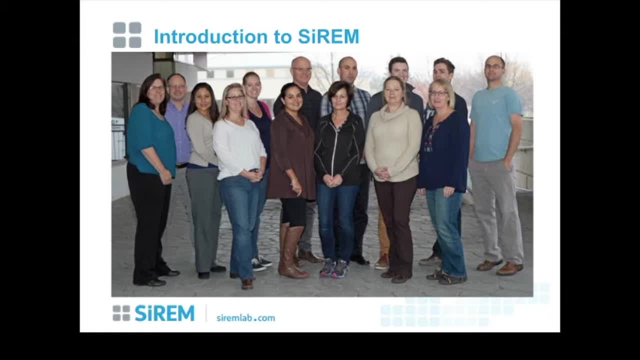 water, but of sediment and of soil. We are located in Canada. We are west of Toronto, Canada, if you know where that is, and a little bit north of Niagara Falls, if you know that, as a landmark in North America. I'm very pleased to be speaking to you today about Serum. 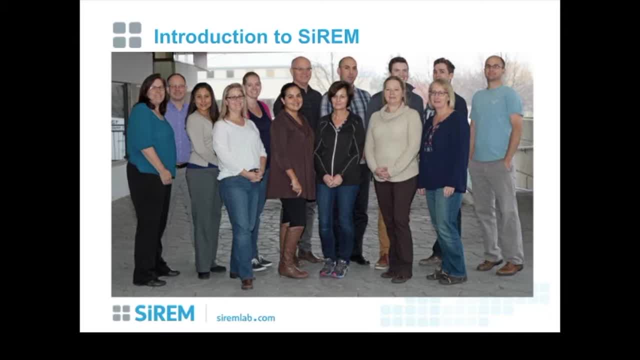 I've been doing treatability studies for Australian sites actually almost from the very time I started doing studies about 15 years ago. so it's dear to my heart, and I've had the fortune of coming over a couple of years ago for the Clean Up Australia conference. so 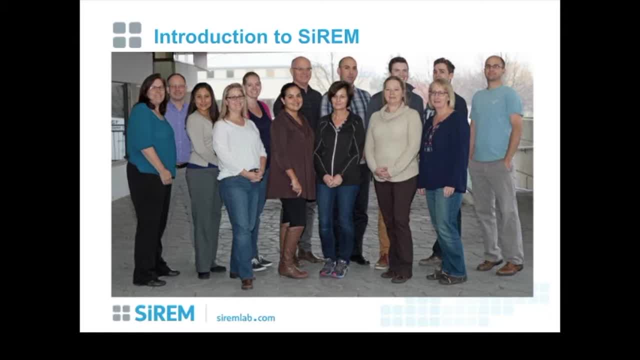 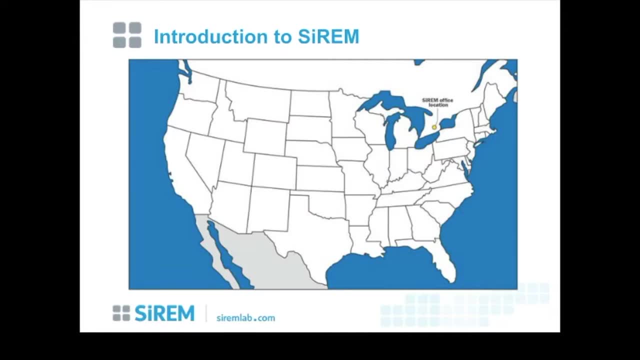 I hope to get back as soon as possible- actually Before our winter's over would be nice, but I'll see when that happens. Here's the map of where we are so you can see in southern Ontario is where we're located, near Lake Ontario, and Toronto is just south of here. 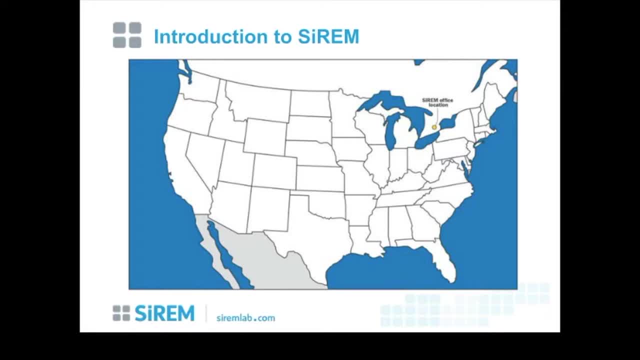 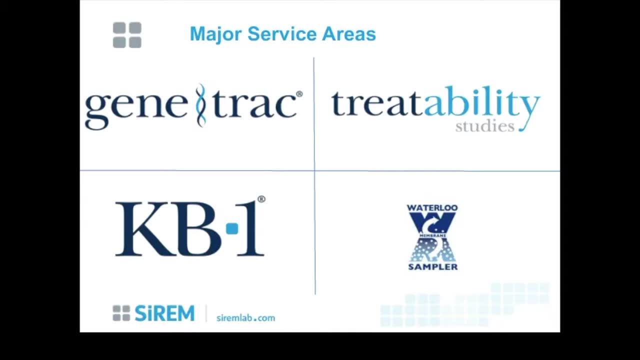 That's the north-east of us. Today I'm going to be talking about our treatability testing services in general, but I wanted to start off first with the products and services that Serum offers. We offer four main service areas: Molecular genetic testing for microorganisms, under the trade name of GeneTrak. 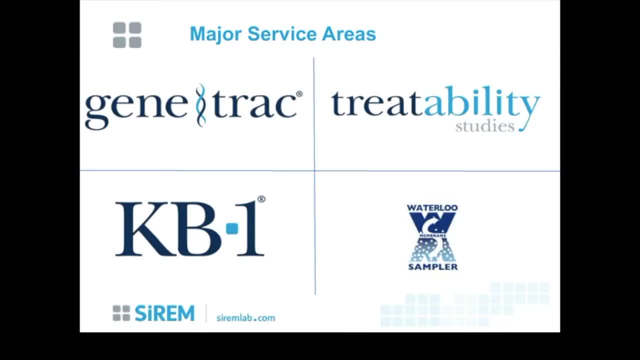 We use DNA-based technologies to identify microorganisms. We have a number of services. We have a number of services. We have a number of services for microorganisms that are known to have specific capabilities related to bioremediation. generally, We offer services that way and we can provide sample filters for DNA extraction and offer. 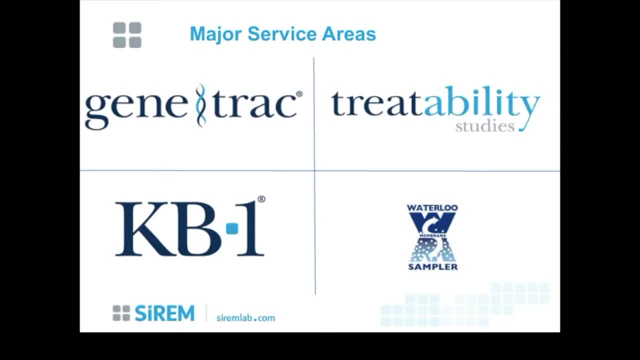 all those services, We have bioaugmentation cultures which have developed from our treatability studies, originally under the name of KB1 and KB1+. These cultures have been widely used worldwide and in fact have been applied in the United States. We have had import permits into Australia and we anticipate actually shipping to another. 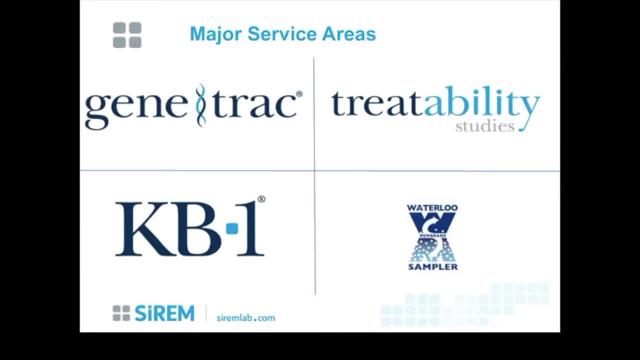 site in Melbourne, I believe in March of this coming year. It's a bioaugmentation culture for degradation of mostly chlorinated solvents in groundwater. I'm not going to touch on it too much, although it will come up in a couple of our treatability. 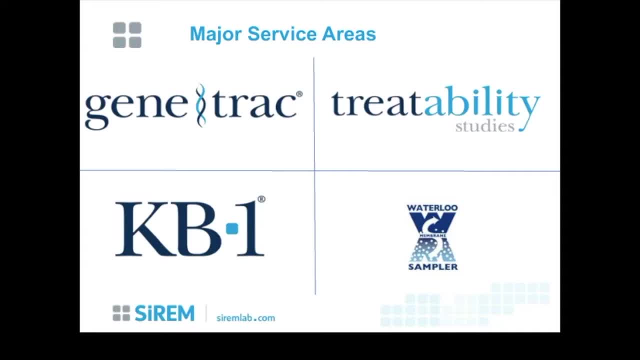 case studies that are being presented. Finally, another product that we sell is the Waterloo Membrane Sampler. This is a passive-diffusive sampler. It's a very good product. It's a sampler used for vapor intrusion applications and if you have interest in that, you can go. 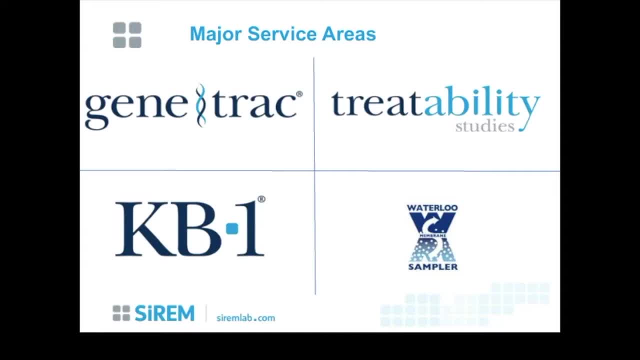 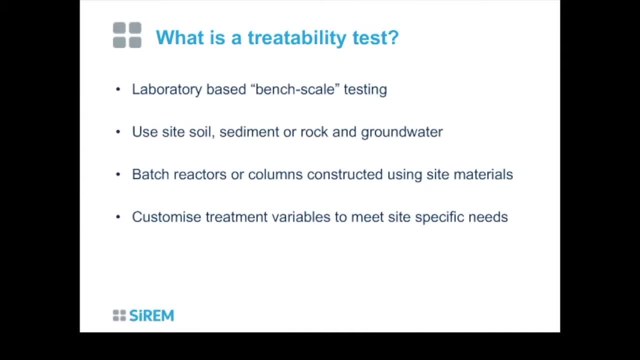 to the serum website and click on the link to the WMS sampler and get more information on that, or send me an email and I'd be happy to direct you to the technical lead for that as well. I'll just jump in here and talk to you. 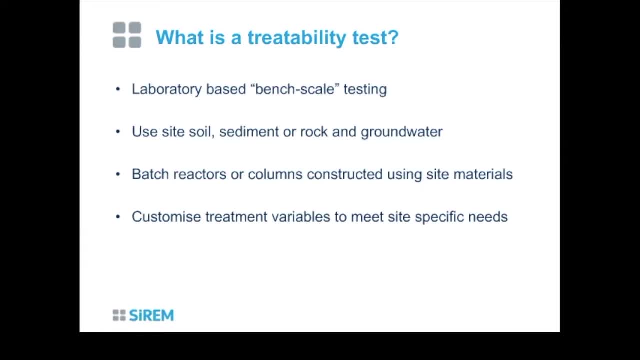 What is a treatability test? Obviously it's bench-tail testing in the laboratory, but we use actual site materials and that's critical that we get That. we get site materials, whether it's soil or geological materials, probably a better. 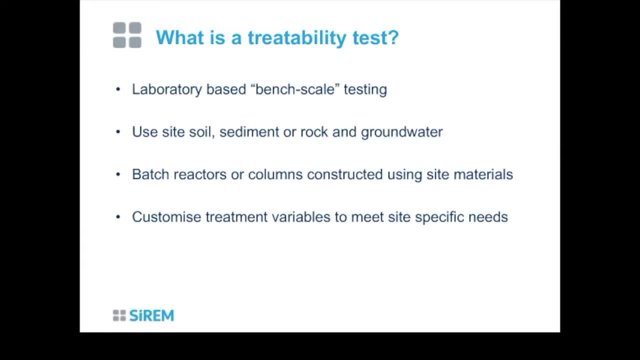 description: sediment, rock and site groundwater and that it comes from the zone of contamination that you're looking at remediating and that's really important that we want to get impacted material, because that's going to be most relevant to testing any technology is we need to have. 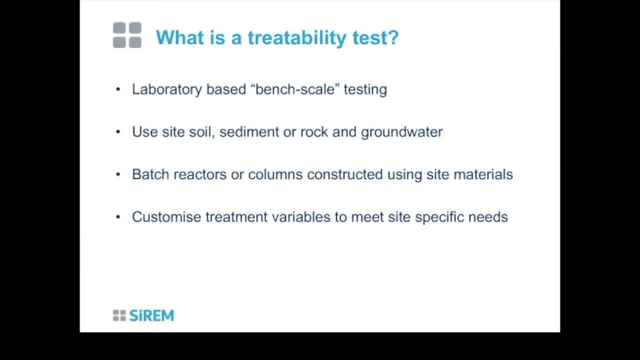 the right matrix to make sure that the technology is going to be compatible with that. It can be done both in batch reactors or in columns That we construct in the laboratory, and they're very customized studies. Although we have a standardized format for a number of our different studies, we customize. 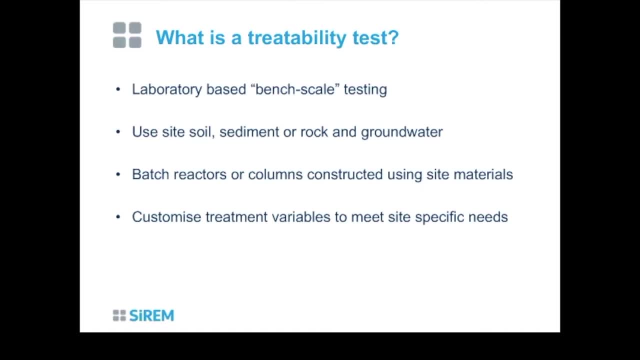 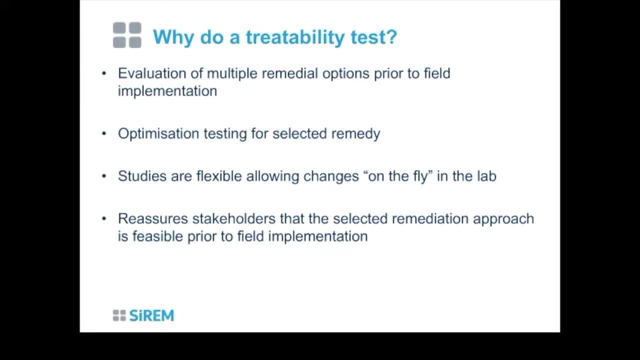 every treatability study to site-specific needs, and so we can address the specific objectives of remedial technology evaluations at sites. A lot of people question clients that don't want to necessarily spend a lot of money. They want to ask: why would you even bother with a treatability test? 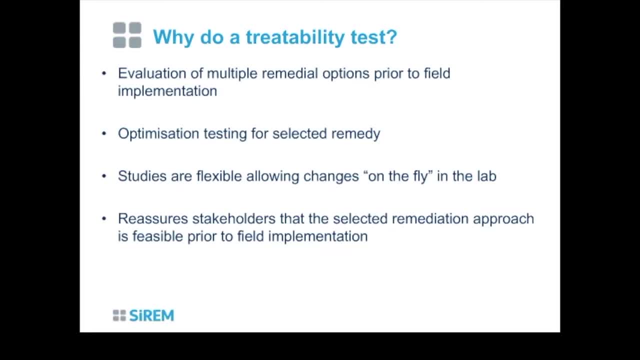 Let's just go right into it. Okay, Let's go right to the field. and one of the main reasons is that you can evaluate a number of remedial options before you get to the field, and you can do it on a cost-effective. 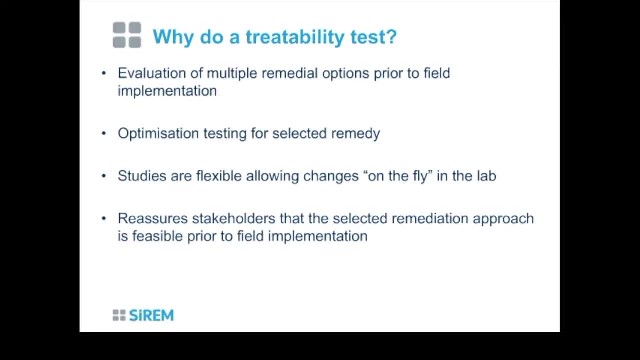 basis in that you can compare ESCO- chemical oxidation versus bioremediation, versus abiotic techniques. You can look at different zones of the site and it allows you to optimize the testing for a specific remedy. so you might do a broad study where you're evaluating general broad. 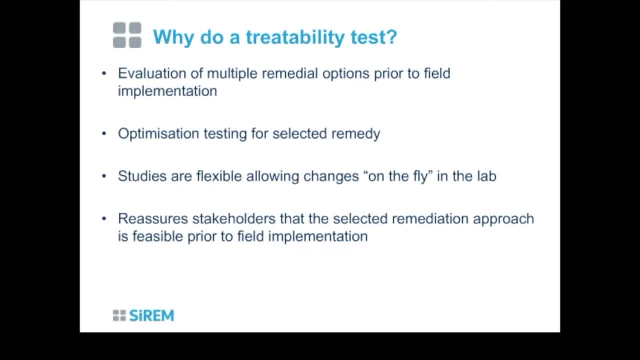 areas, Maybe three or four different oxidants perhaps, but then you can then also do a more specialized study that hones in more specifically on what type of electron donor might you want to apply or work best at the site? what oxidant activation chemistry might work? 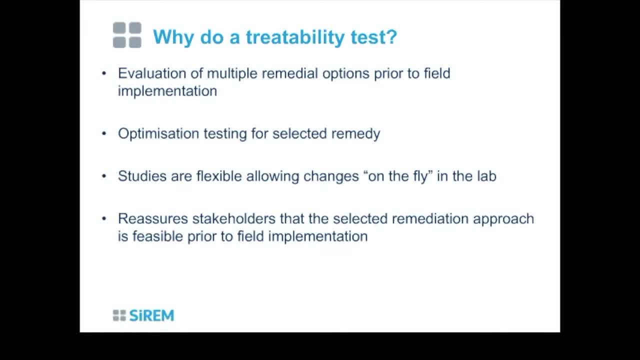 Our studies are very flexible in that we can get relatively fast turnaround time on analytical data. that allows us to make changes to the scope of the study without making huge changes in the cost of the study, because if a study is designed with a certain number of sampling, 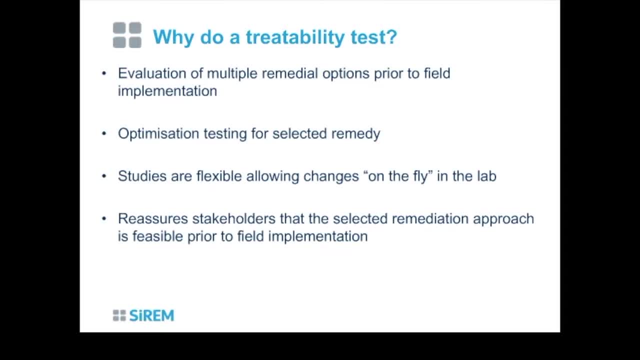 events, that cost doesn't change If we make one small change to a treatment, or what we call a change on the fly. it doesn't impact the cost at all, and so we can be very flexible and change direction If something isn't working or something's working faster or slower than anticipated. 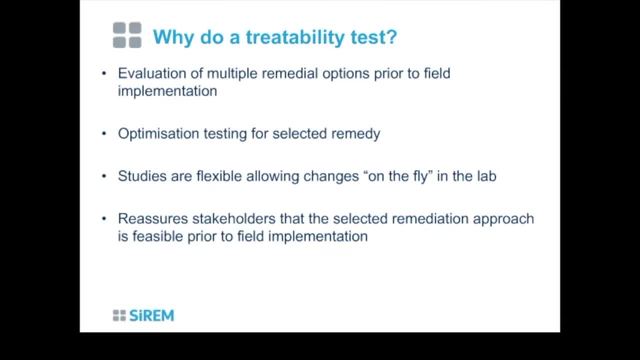 we can address that immediately so that we can get the best output of results in time for development. We can just continue working from that point forward. I want to just kind of want to refer back to this like part of the summary and maybe take you through a couple more slides. 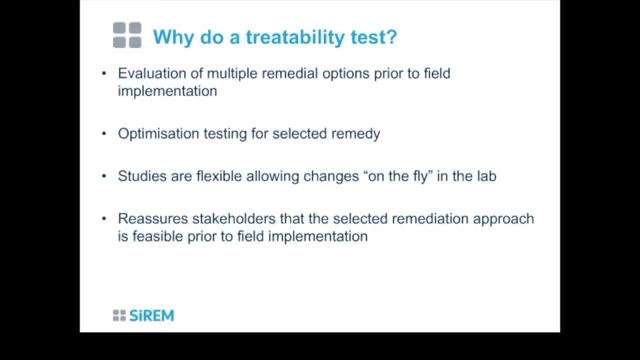 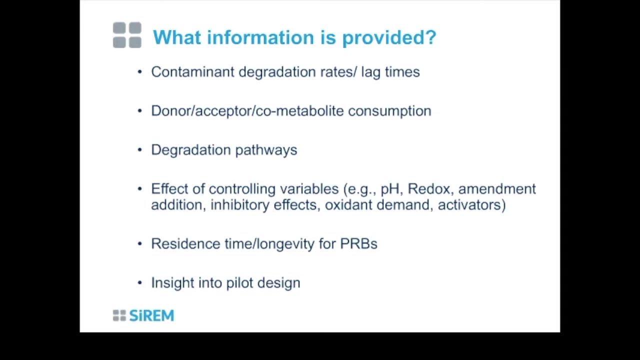 As we go through this kind of as the general ihr� and then the second part, as we get to the end, we'll just sort of lower the threshold and we'll get back to the bigger picture. We're going to look at the relationship between the patient and the program and then we're 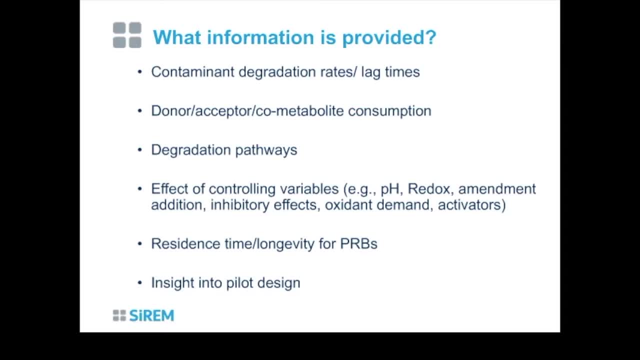 going to look at the relationship between the patient and the program and then we're going to examine both of these Very obviously. you're going to get contaminant degradation rates. Is benzene going to be degraded? Is tricloroethene going to be degraded? 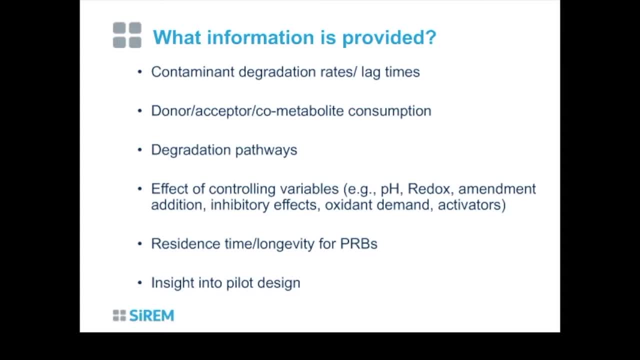 Is what intermediate products are going to be produced. You can get information on amendments that you might add, whether it's an electron donor or an electron acceptor or a co-metabolite that you're adding. You can get some idea of how fast they're being consumed. 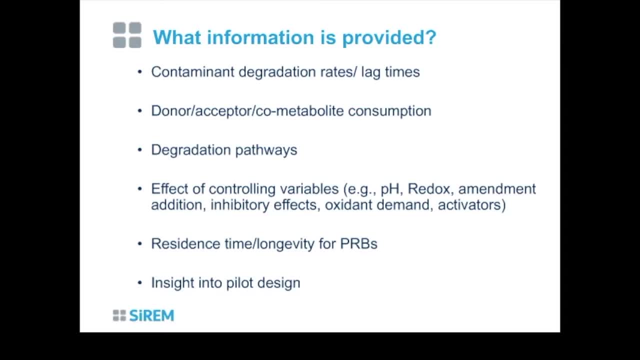 In some cases, you can get elucidation of specific degradation pathways if they're not already well-known. And, very importantly, you can look at the effect of controlling variables, which can be very significant at some sites where you don't realize something has a stronger effect than you anticipated. 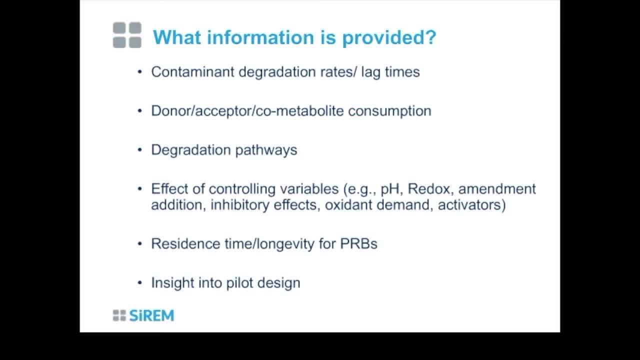 pH and redox are very, very important, as well as contaminant mixtures. Individual contaminants may be able to be degraded in the long run. You can see that in the laboratory, But the mixture testing in the laboratory is more important to understand as well. 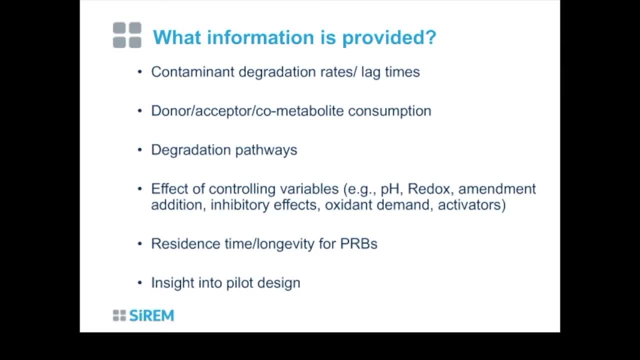 If you've got chloroform present with chlorinated ethene such as TCE and PCE, you need to understand what that means and what that might affect a bioremediation application For using permeable reactive barriers, often with zero-valent iron or a ZVI. 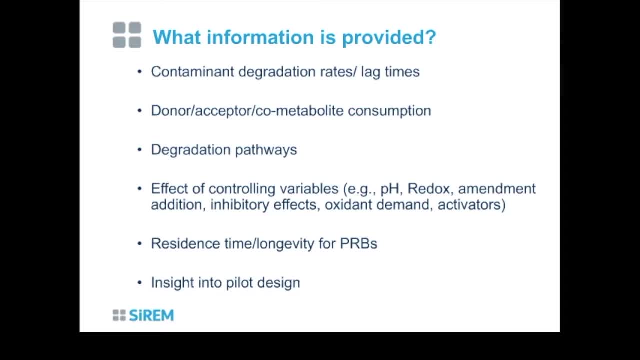 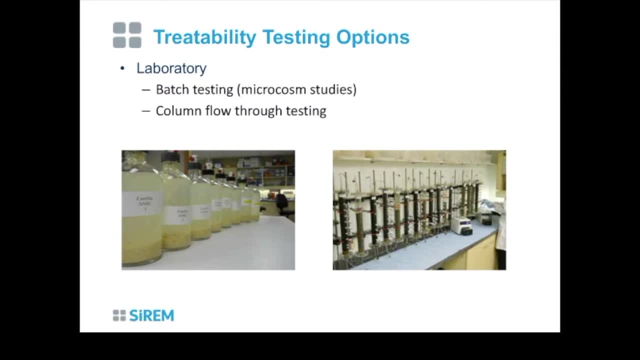 you can get information that provides design, information that allows you to design the resident time and longevity of a potential barrier application. So just a couple of visuals from pictures in the lab We put dirt in bottles. That's a lot of what we do. 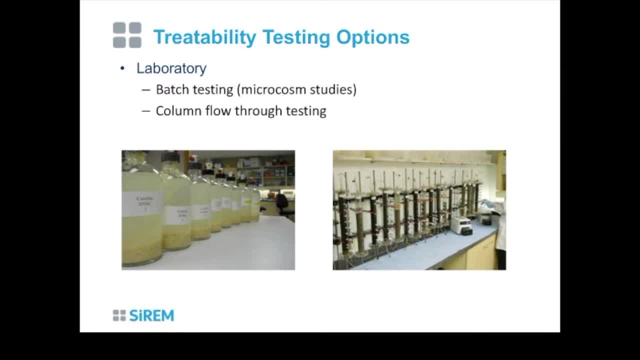 And we use sacrificial or continuous batch testing which we call microcosm studies. So there are some pictures with some very unusual-looking site geological material in the picture here, sort of a side view along those bottles before they got put in the anaerobic incubator. 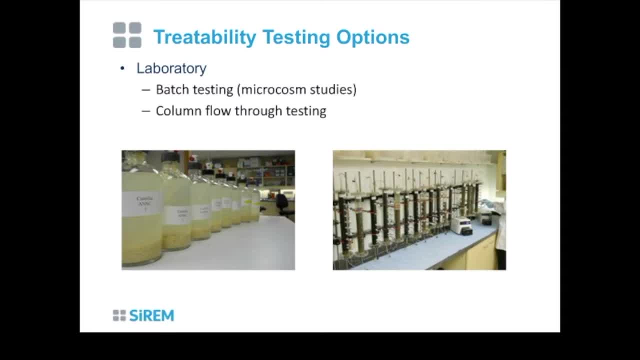 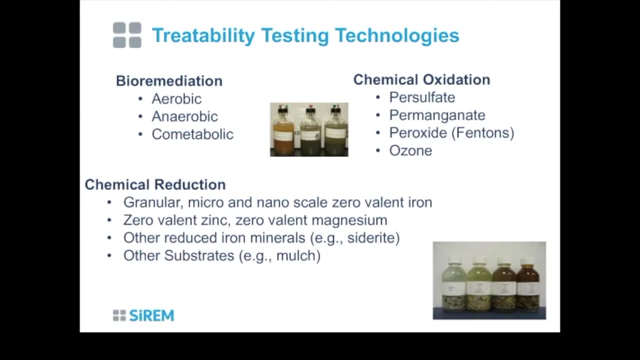 as well as on the right-hand side, As well as on the right-hand side here- a set-up of all our column studies that we have in the laboratory, And so the two main areas are batch testing and column flow-through testing. The types of treatability technologies that we can test in the laboratory are limitless. 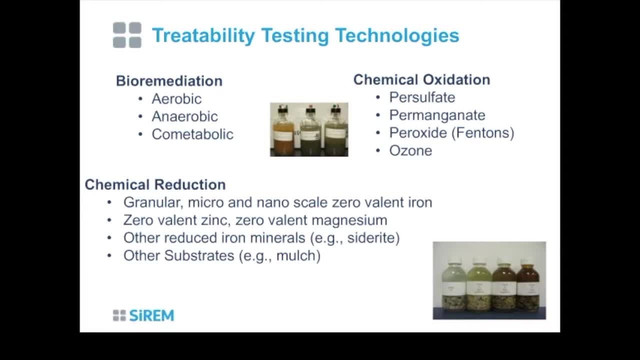 Generally they fall under three main areas that we typically evaluate, but they can really be used to any sort of technology that you do want to test. So for bioremediation applications, most often you're looking at either aerobic or anaerobic or co-metabolic applications. 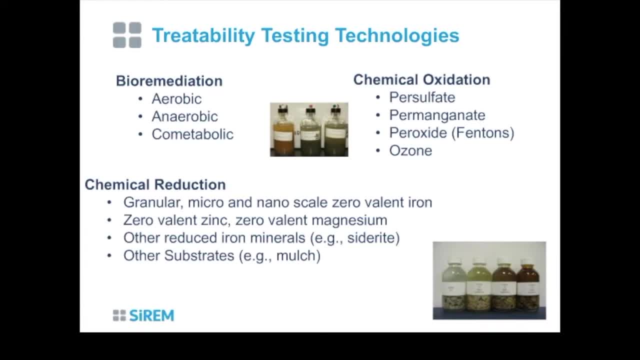 For chemical oxidation. we have extensive experience with persulfate permanganate and a little bit of experiments with peroxide and ozone. They're a little bit more volatile and challenging compounds to work with in the laboratory, but we have conducted them with some success. 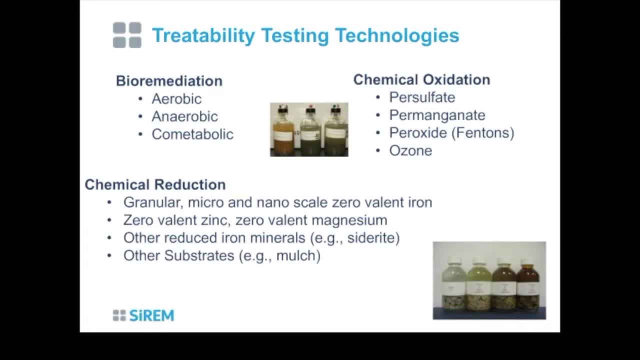 We can do oxidant demand, We can do treatability of actual compounds with the different oxidant chemistries that are available, And we often use reagents directly from vendors. So we want to use the reagent that's going to be applied in the field. 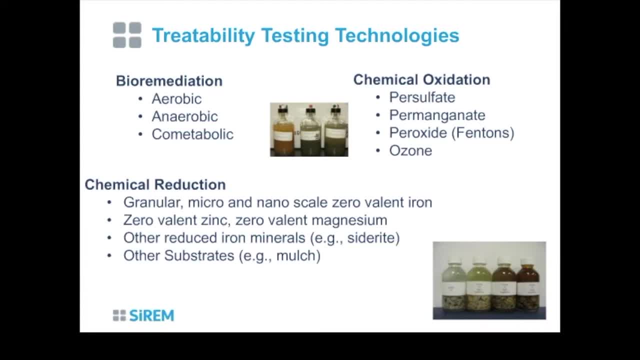 So we'll try and obtain reagents right directly from a vendor that you might be using at a site, so that we're testing the right material. Chemical reduction studies typically involve evaluation of zero-valent iron, or ZVI, in various different scales, and other bimetallic metals that also can be tested. 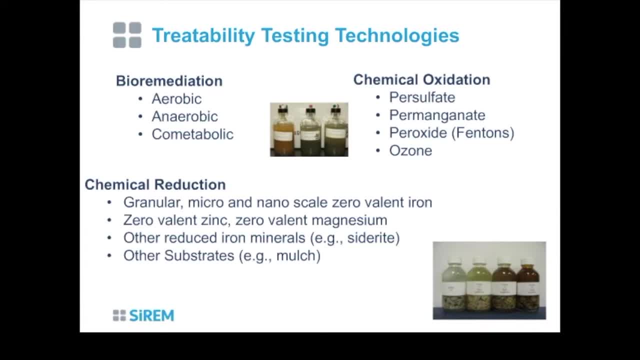 And other things, such as reduced iron, minerals such as siderite, or other substrates such as mulch, which is often used in bio-barriers, And this testing can be done in the different media that you have available to us, whether it's the site, soil or geological material, ground water, waste water, surface water. 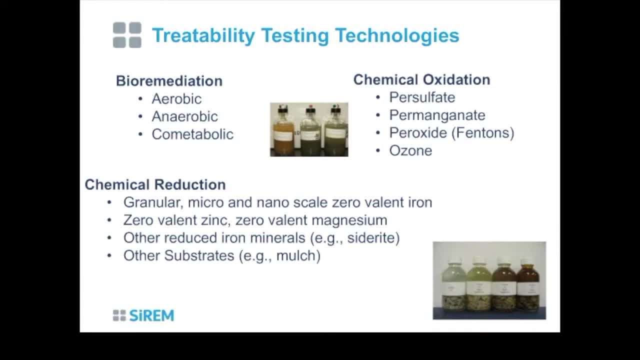 sediment, pore water. All of those things can be tested in the laboratory. Some of them are a little bit more challenging to get, samples of pore water in particular, But most everything else, it's easy to get the samples to be tested. 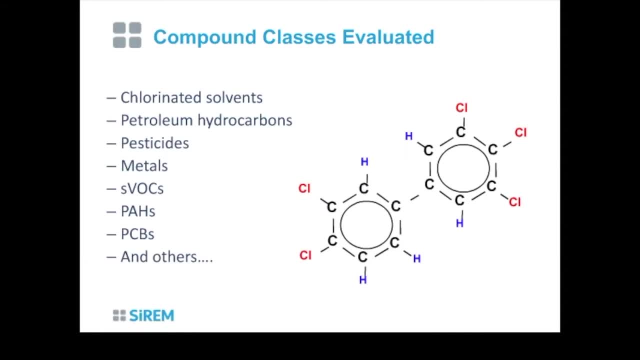 The compound classes that can be tested in the laboratory also are limitless as well. We started off really getting our experience with chlorinated solvents about 10 to 15 years ago. We did a lot of treatability studies with trichloroethene. 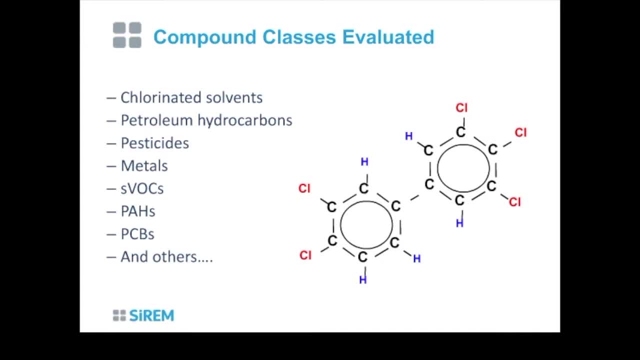 and looking at biodegradation with the Helicoccoides organisms, But that's since been expanded to a wide variety of different chlorinated solvents: chlorinated ethanes, chlorinated ethanes, chlorinated methanes, chlorinated propanes. 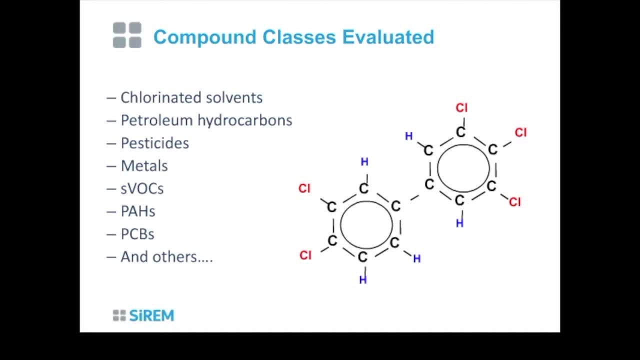 various petroleum hydrocarbons, pesticides, whether they're chlorinated or not, inorganic metals, and the list goes on. And much of that can be analyzed in-house in our laboratory, which is also what helps us control our costs of our studies. 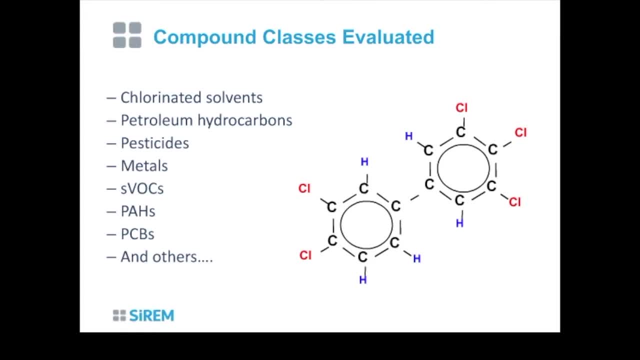 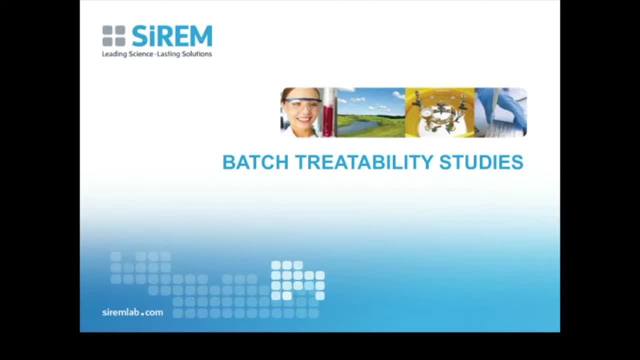 as well as we use local and regulatory approved analytical laboratories for some of the compounds that we don't analyze in-house ourselves. So now I'm just going to focus on how we conduct our batch treatability studies and give you a little bit more further information on those. 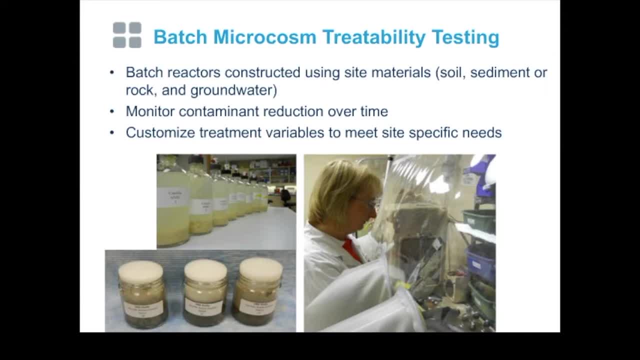 So, again, as I said, we construct them using site materials that you get from the zone of contamination, And what we typically do is we monitor contaminant reduction over time And again. we customize the treatment variables to meet your site-specific needs. 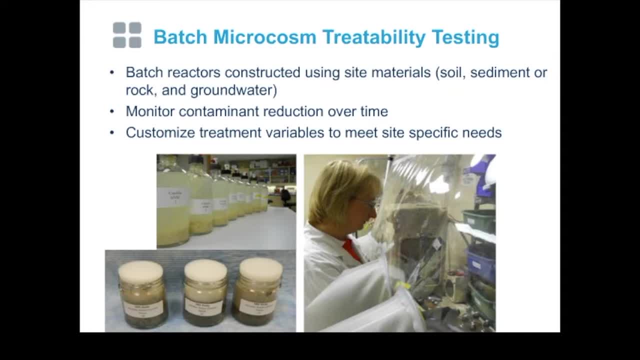 And in the photographs here again the bottom. here we have some petroleum hydrocarbons where we just have an equivalent of vatosone soil with aerobic treatment. So you have these soil stoppers that are placed in these wide mouth bottles with a lot of air exchange that can be allowed through there. 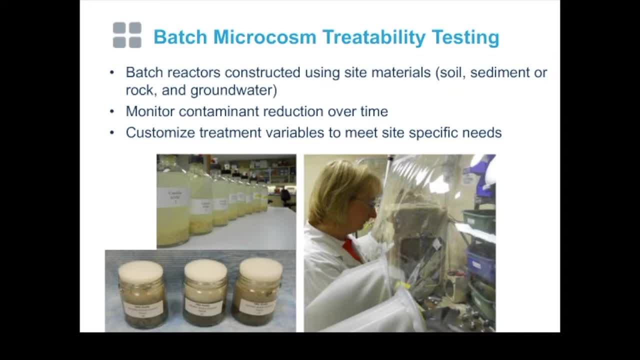 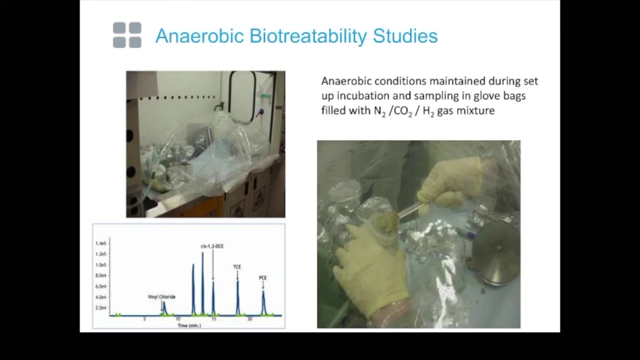 and looking at seeing what degradation you get in the soil phase. On the right-hand side of the picture is one of our anaerobic chambers where we incubate anything that needs to be kept under anaerobic or reducing conditions When we get the materials from the site. 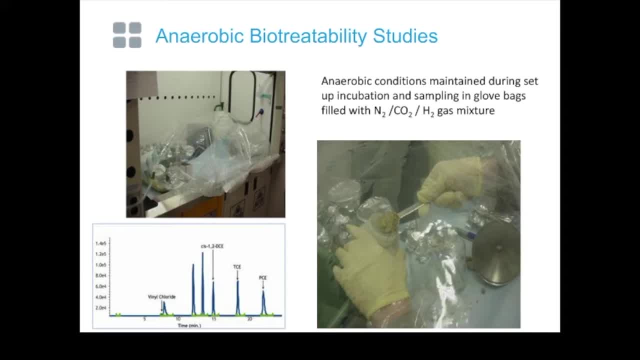 we actually set up all our microcosms in chemical fume hoods. We've got the sash all the way up in our fume hood, just so we can take a picture here. We put all the materials into a temporary anaerobic glove bag. 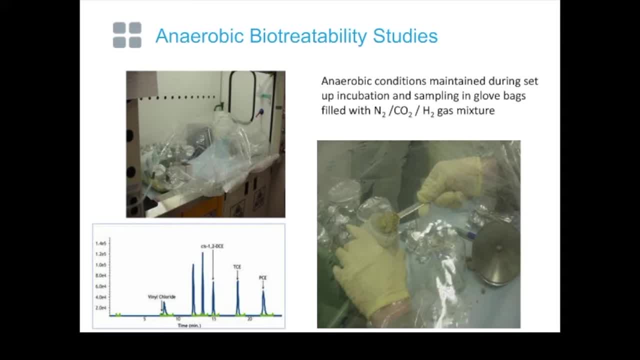 These have arm holes in them here so that you can put your arms in. We remove the soil or the geological material from the cores and homogenize it. We have the groundwater in these carboys here that are typically 4-litre size. 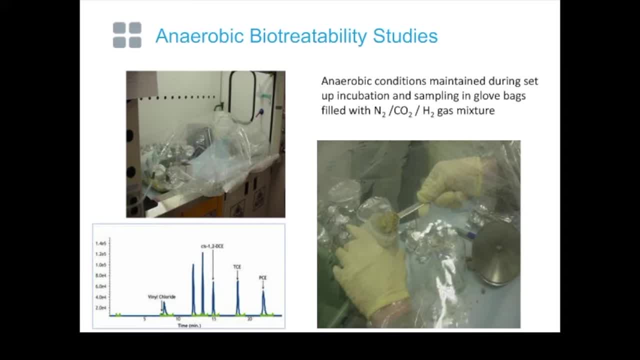 We measure out the soil, either volumetrically or gravimetrically, into sterile batch bottles, add the groundwater to them, all done for anaerobic studies under a gas mixture that keeps it anaerobic, or if it's aerobic, we'll just do it in the ambient air. 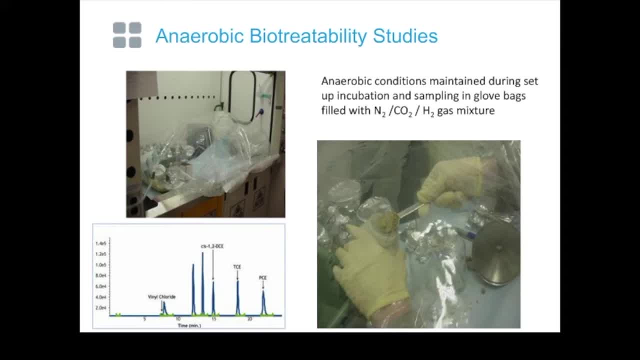 And again, it allows us to set up these studies with no cross-contamination. So one study per disposable bag. the bottles are all set up and they're capped and then they're transferred to the appropriate incubator, which is, for anaerobic studies, an anaerobic incubator. 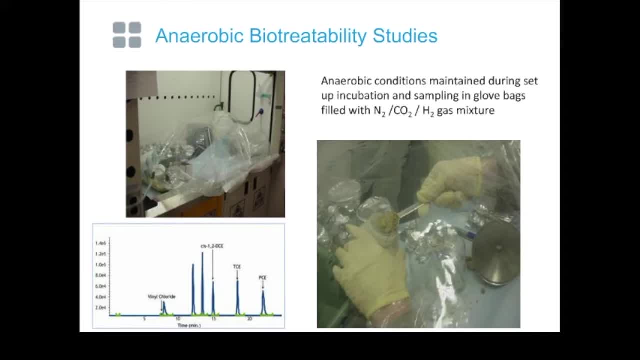 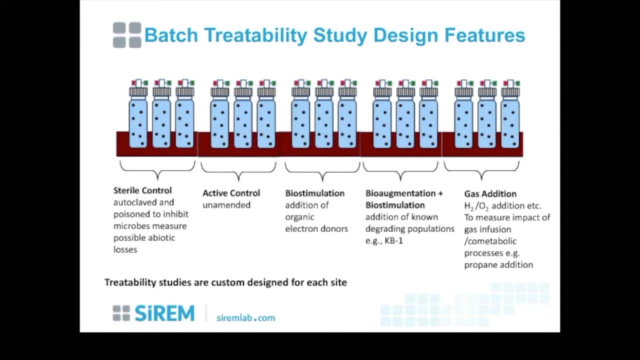 For aerobic studies it's just room temperature out in the laboratory. So this cartoon here just is a really good demonstration of how we design our studies, And one thing that we stress is replication. So most of the time, with some exceptions, we run everything in triplicate. 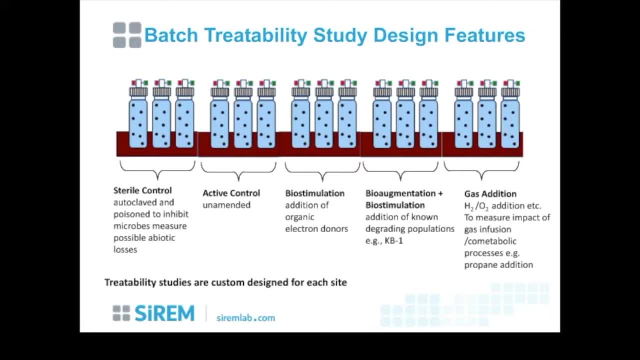 And we find that triplicate. reactors just allow us enough information about the variability of the data that you can trust things And that duplicates. if you have one go one way and one go the other way in terms of results, you don't know which one's the right word. 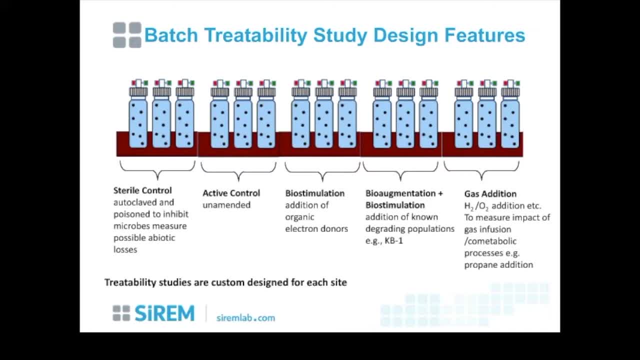 With triplicates you get a measure of the average and the standard deviation and over time you get a really good understanding of the trend. We typically have controls for batch studies. For a biological treatability study, we'll have what's called a sterile control. 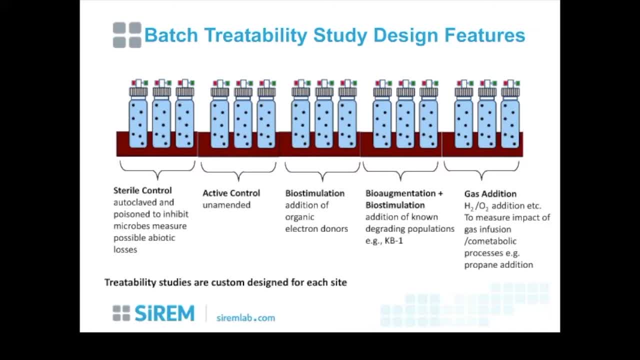 where the soils are autoclaved and poisoned and the groundwater is poisoned to inhibit microbial activity And also so that we can measure any abiotic and experimental losses. So any losses that might occur due to absorption or due to sampling variability can be measured in a sterile control. 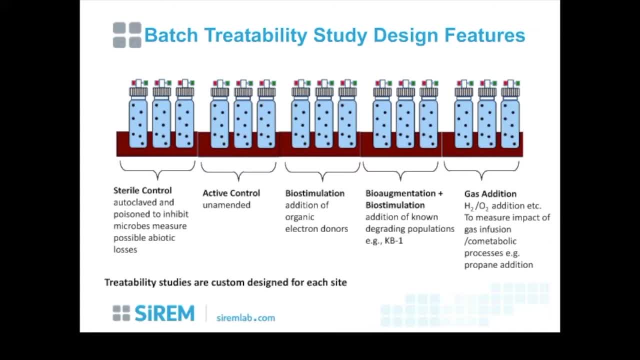 What we call an active control or an intrinsic control is simply just natural attenuation. We're not doing anything to those, We're not adding any amendments, We're just sampling it over time and seeing what happens, whether abiotic or biotic, And then we can look at, especially for treatability studies, where you're looking at biomediation. 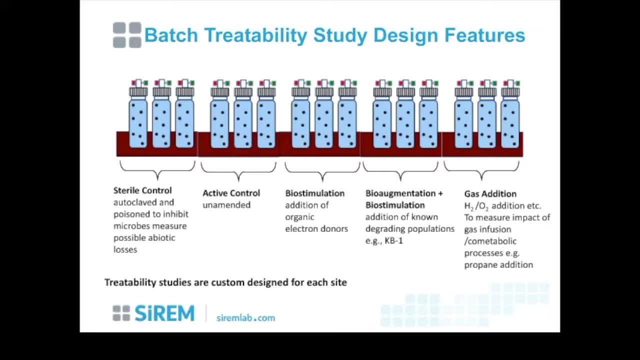 you're looking at biostimulation, where you're adding either electron donors or electron acceptors and looking at biostimulating. So basically you want to see if indigenous microorganisms can be stimulated in their activity just by the provision of food. 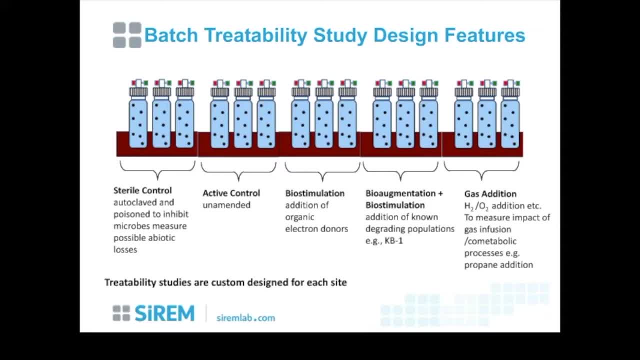 And you can also try other nutrients that might be added as well. Supplementally, we know that some sites don't have the right microbial populations for development, So you want to look at that as well, And then we can look at biodegradation. 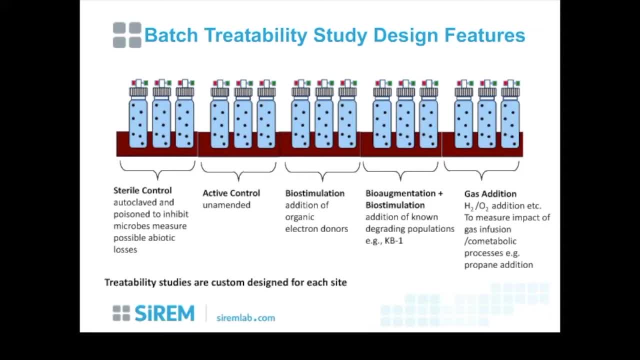 And so bio-augmentation cultures can be added to the microcosms and tested as well, And typically for anaerobic studies you don't add bio-augmentation cultures until reducing conditions are achieved, And for aerobic and co-metabolic studies we can add various gases to measure the impact of gas infusion. 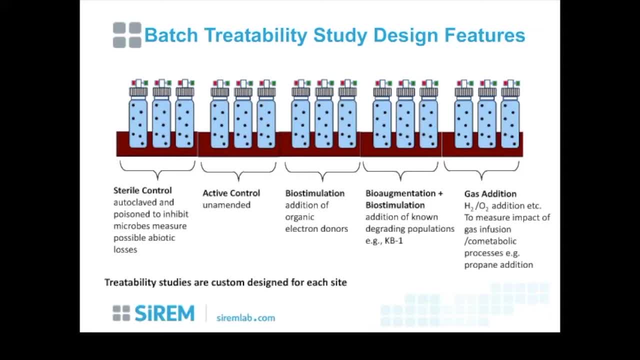 as well as the impact of co-metabolism. So for aerobic 1,4-dioxane co-metabolic degradation, we can look at using various alkane gases to promote co-metabolic degradation of 1,4-dioxane. 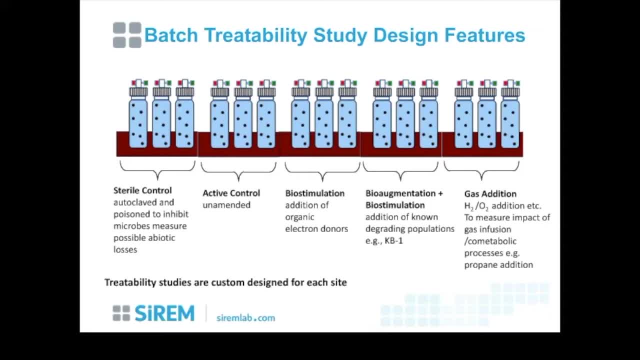 And often for petroleum hydrocarbons. aerobic studies are quite often used to look at aerobic degradation of benzene BTEX compounds. Again, we must stress that our studies are custom designed for each site, So some sites might not want to look at bio-augmentation, and we take that one out. 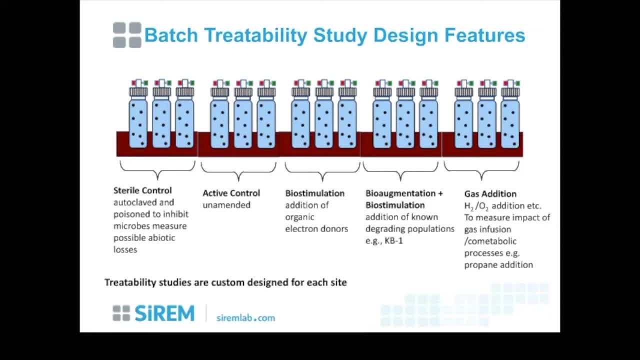 We may want to have additional controls. Perhaps we're going to adjust the pH. There's a variety of different things that can be adjusted and that is usually at the proposal stage. We go through the site data with you when you're looking at trying to understand what you want to do for a treatability study. 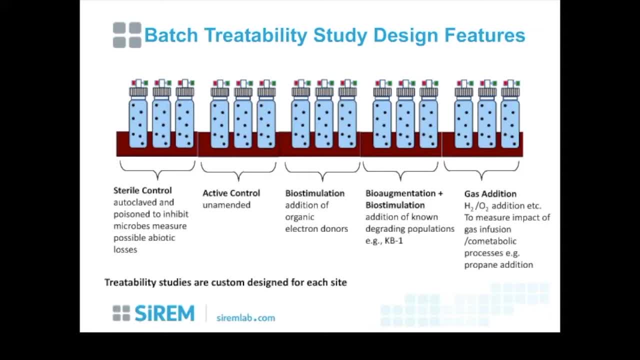 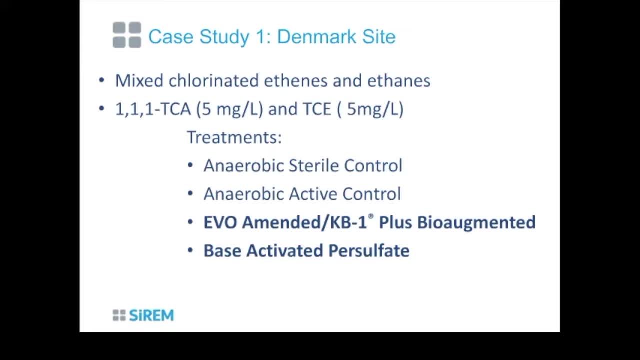 and work that out right at the proposal stage. I'm going to jump right now into a case study. This site's in Denmark And the contaminants of concern are 1,1,1-trichloroethane or 1,1,1-TCA, and trichloroethane or TCE. 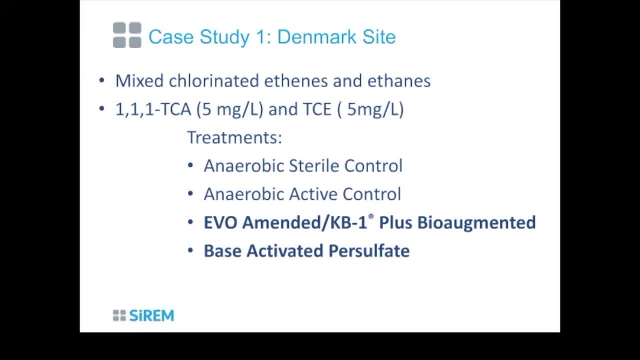 And the client objective of this study was to compare both bioremediation and in-situ chemical oxidation, And so this first part that I'm going to present is some of the biology bioremediation results, and then I'm going to show you the base-activated prosulfate. 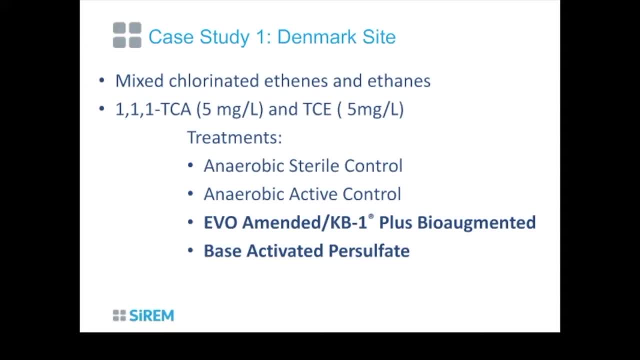 I'm not going to show the results of the sterile control and the active control in the interest of time. I will have another case study that does show some control data so you can see what you get in those types of results. So the first treatment that we looked at was an emulsified vegetable oil, amended. 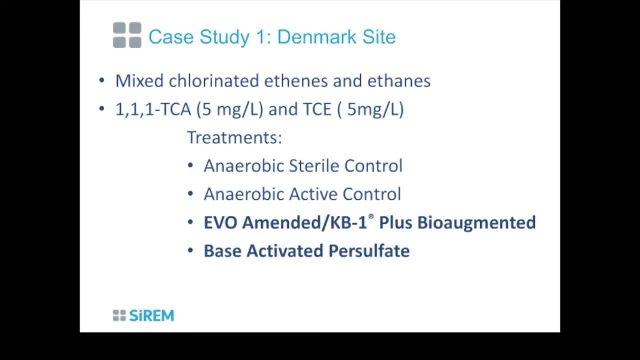 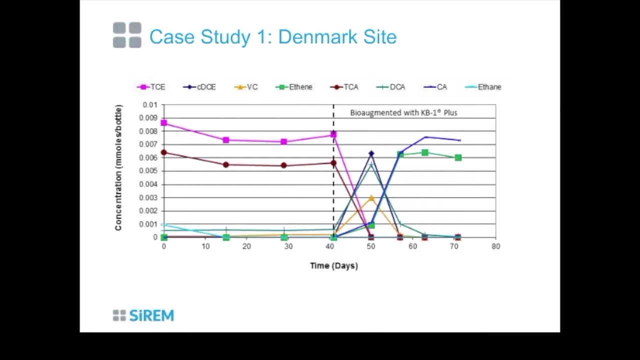 and a bio-augmented treatment, and that's EVO is for emulsified vegetable oil, And both contaminants were at about approximately 5 milligrams per liter in the aqueous phase. So here you see the results presented in millimoles. 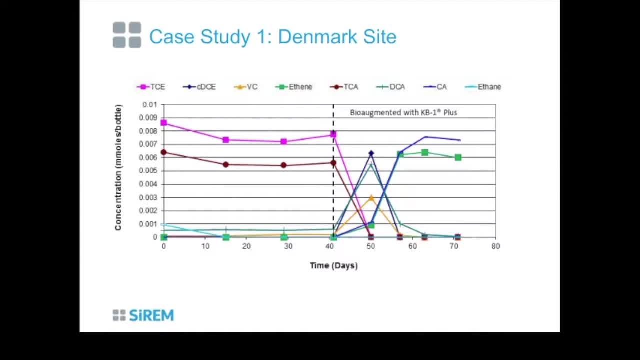 So we've taken the concentration data and looked at the total mass of the contaminant in moles per bottle. It allows us to look at mass conversion in bioremediation applications. You can actually see really good mass conversion, so it's a nice way to visualize the data. 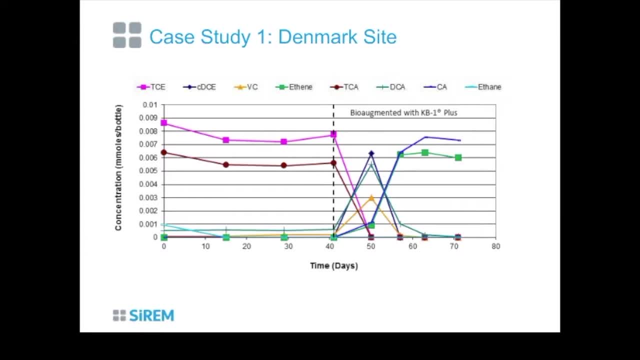 TCE is in the bright pink color. 1,1,1-TCA is in sort of the reddish-brown color And you can see for the first 40 days of incubation where it was incubated with an emulsified vegetable oil. 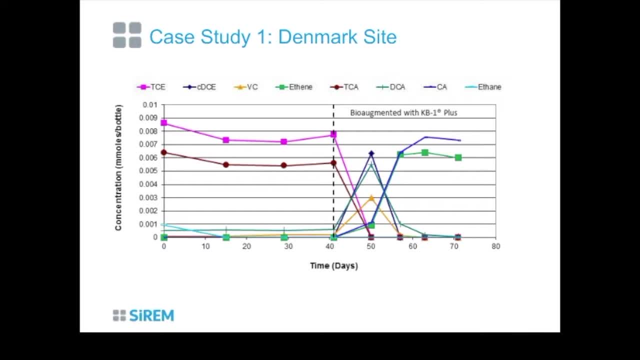 under anaerobic conditions. not much happened. We didn't really see anything move at all. So at day 41, we bio-augmented and what we saw was rapid and complete dechlorination of the 1,1,1-TCA to chloroethane and the TCE to ethene. 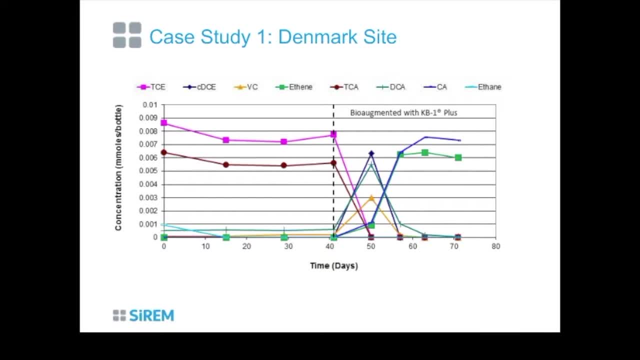 which is very typical for the bio-augmentation cultures that we have available, And it also shows really nicely the dechlorination sequence. So you see TCE in pink going to silver, Cis-DCE in the dark blue Going to vinyl chloride in the orange. 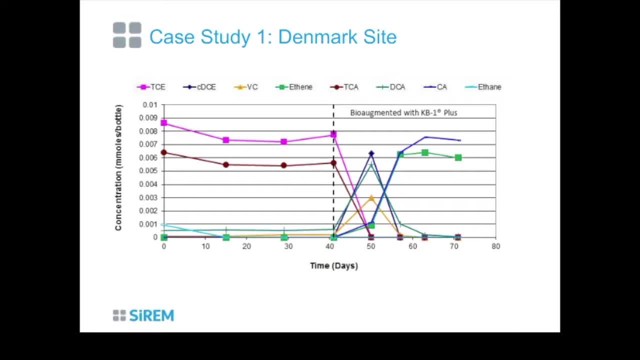 And then ultimately to ethene And you can see fairly nice mass balance with the amount of TCE that we started off with And then the TCA degrading from the red to 1,1-DCA, which is the turquoise under here. 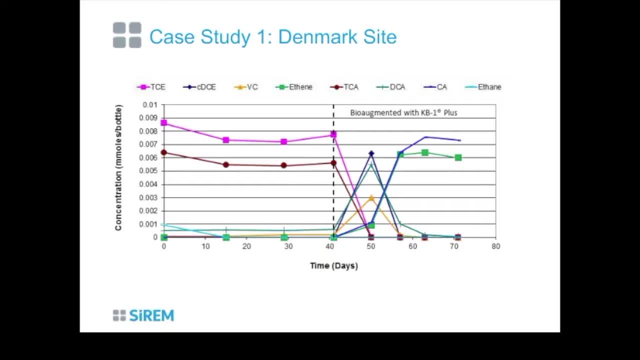 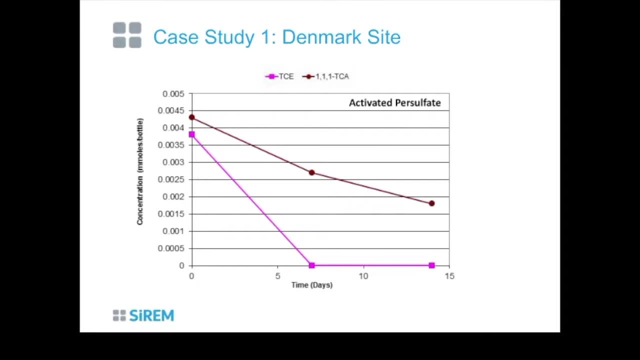 And then going to chloroethane. Chloroethane is not further degraded under anaerobic conditions, but then can be degraded under aerobic conditions. And here are the results from an activated persulfate treatment And what we saw is this is a much less intense study. 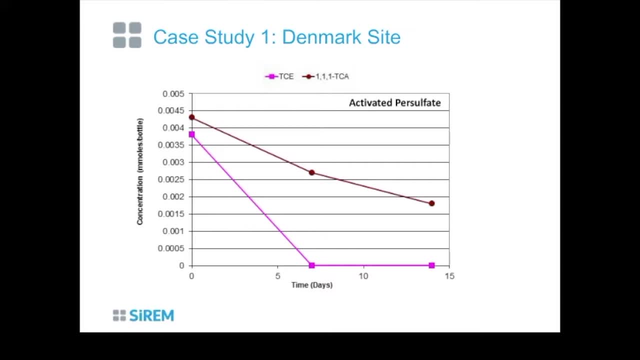 We just did a quick snapshot after 14 days- And oxidant studies are typically very fast moving and very quick- And what we saw was that all the chloroethanes were degraded by seven days, very rapidly and as expected, And that 1,1-TCA wasn't as rapidly degraded. 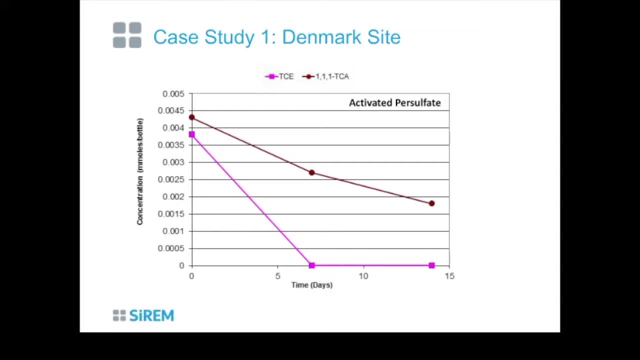 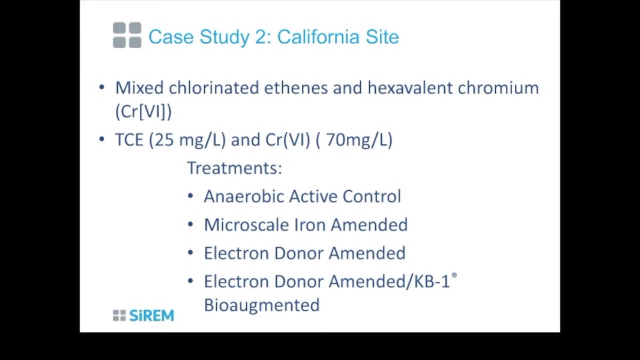 nor did we see complete degradation with the consumption of the persulfate. Ultimately, the client went to the field with the bio because it was the best option to treat all the contaminant classes. The next case study is a site in California where we are evaluating a bioremediation approach. 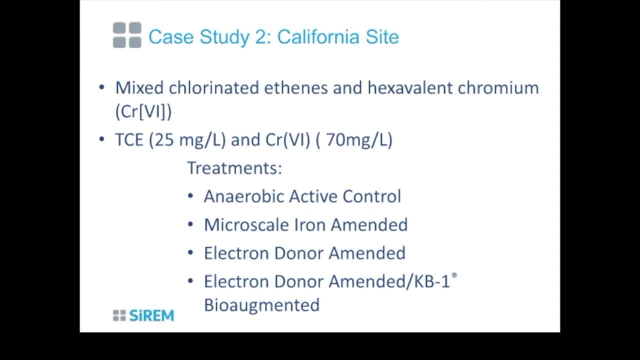 versus an abiotic degradation with zero-valent iron, And what we looked here was with trichloroethene at 25 milligrams per liter, which is pretty high for some sites, and hexavalent chromium at 70 milligrams per liter. 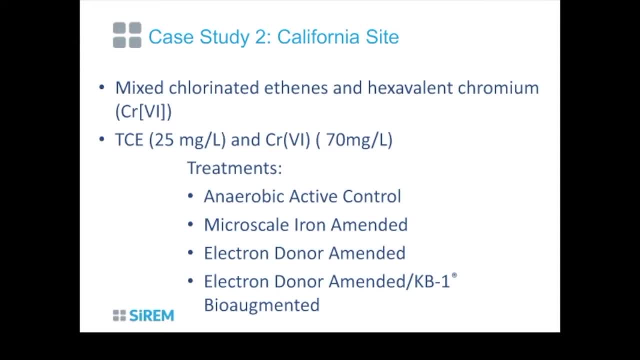 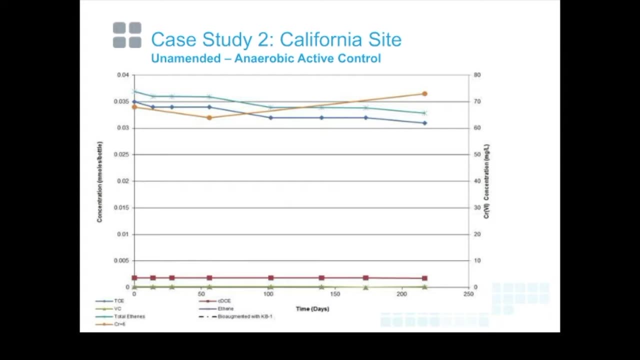 And the treatments that we assessed here were intrinsic degradation with an anaerobic active control, micro-scale iron- looking at the CVI application- and an electron donor with and without bio-augmentation. So here's a really nice control. The study ran out a pretty long time. 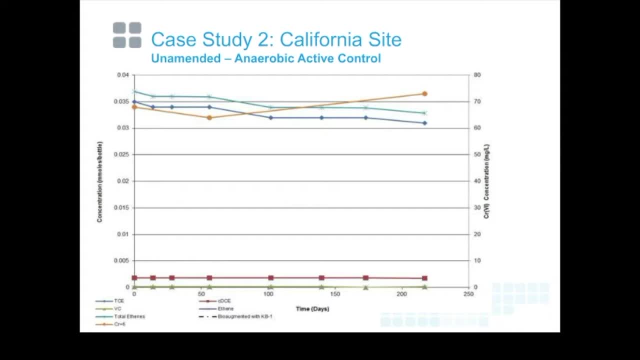 You can see it ran out over 200 days And you see the main contaminants. We have hexavalent chromium and that's in concentration in milligrams per liter On the right-hand axis here And we have the chlorinated ethynes in total millimoles. 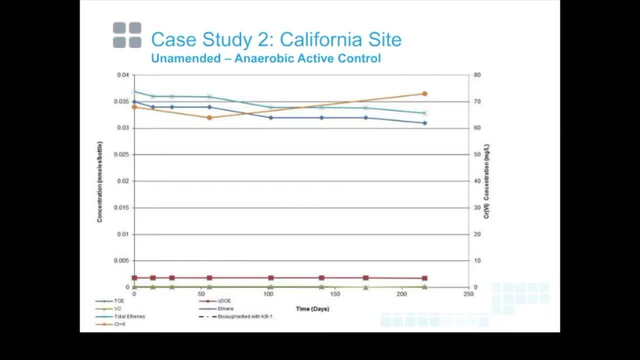 on the left-hand axis And you see that the TCE showed a very small decline over the incubation period. That's within the normal experimental variability of 10 to 20 percent is pretty standard for analytical and experimental variability And we don't see any significant changes in those over time. 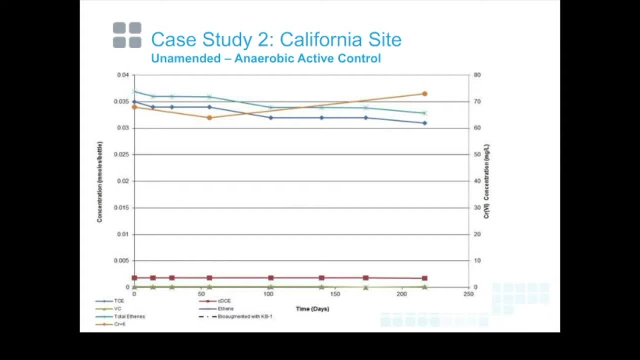 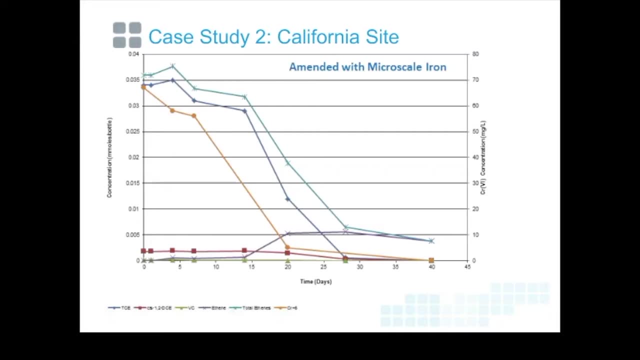 And you see that the total mass of chlorinated ethynes is pretty consistent as well. So in the treatment amended with micro-scale iron, you see very rapid degradation. One thing to point out was that the hexavalent chromium was so high that the water was yellow. 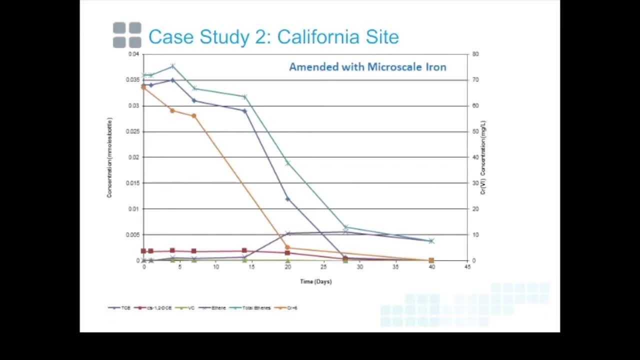 So it was pretty toxic water And what we saw, amended with iron, is we saw the hexavalent chromium drop out very quickly and down to non-detect concentrations within 40 days. We saw the chlorinated ethynes, the TCE, drop out. 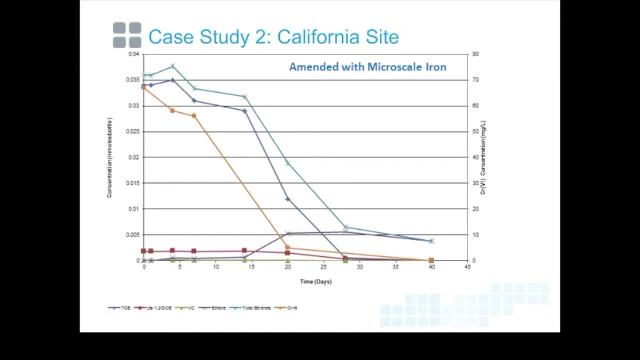 and the cis-DCE drop out between day 25 and day 30.. We saw very little production of ethyne, which is a typical result with ZDI. You often get acetylene being produced, so you're getting contaminant destruction all the way to acetylene, ultimately CO2.. 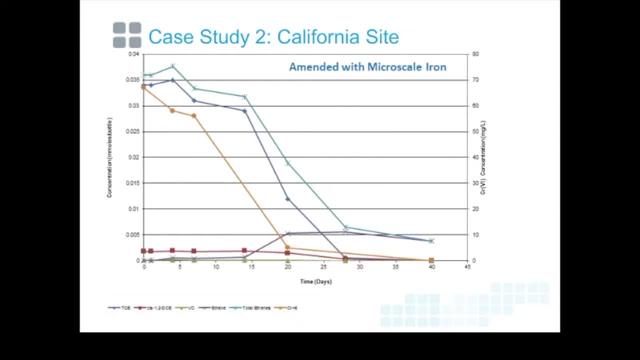 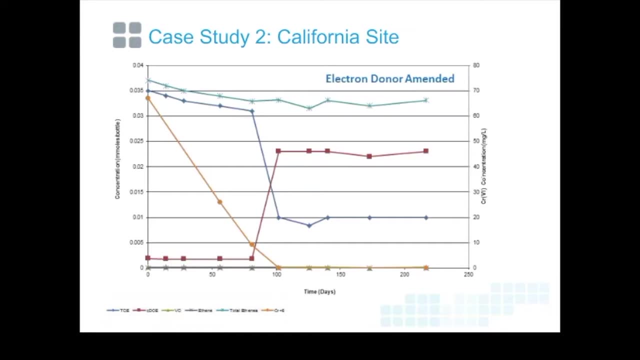 And so you lose all your mass, and that's a great result. there The electron donor treatment shows very clearly we get some degradation with the amendment of electron donor. What we see is hexavalent chromium dropping out pretty rapidly by day 100. 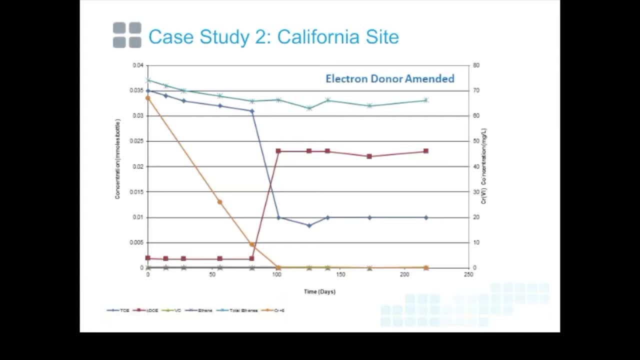 And that we see TCE. once the hexavalent chromium was significantly reduced, we saw TCE being degraded to cis-DCE, But then, after day 100, for the next 100-plus days, we didn't see anything happen. And so when we now look at our bio-augmented treatments, 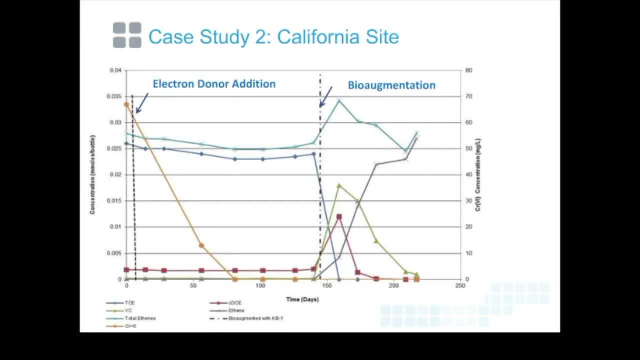 it's exactly the same as the previous treatment, with the exception that it was bio-augmented just before day 150. And you can see the same results as before. Initially hexavalent chromium dropped out. We didn't actually see the TCE go away at all in this treatment. 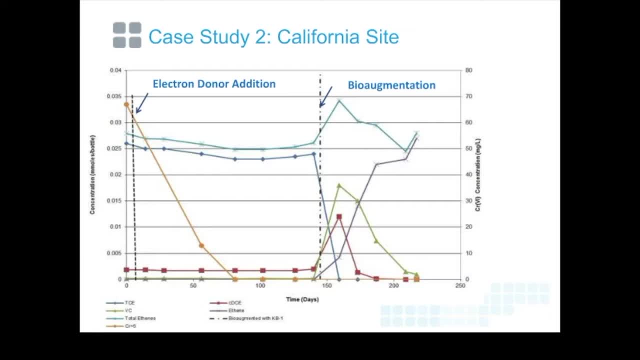 Once we bio-augmented, then we saw cis-DCE and vinyl chloride being produced, with the production ultimately of ethyne being produced and a good mass conversion of all the moles of TCE were converted to ethyne, which is very typical for chlorinated ethyne bio-augmentation. 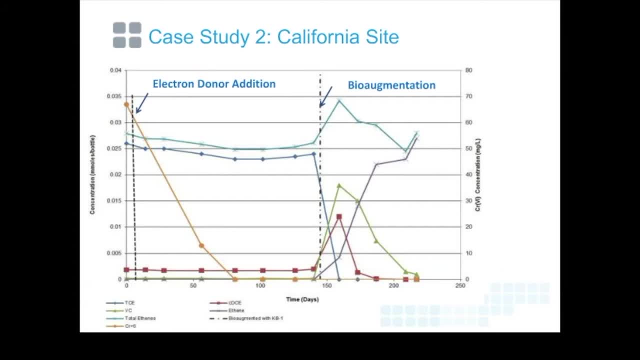 And so we can see the same results in the bio-mediation sites. So in this site- sorry, I'll go back to that slide for one moment Again- the client went to the field with the bio-mediation approach and they did observe very similar results. 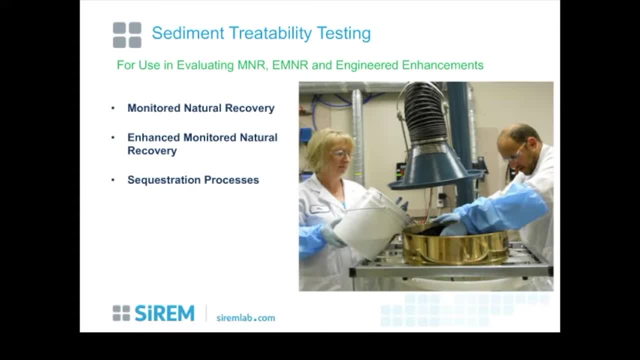 to what they saw in the treatability study, Sediment treatability testing. this is just sort of a placeholder to say that we can do a lot of treatability testing very similarly to the sediments applications. The terminology is often different than for bio-mediation. 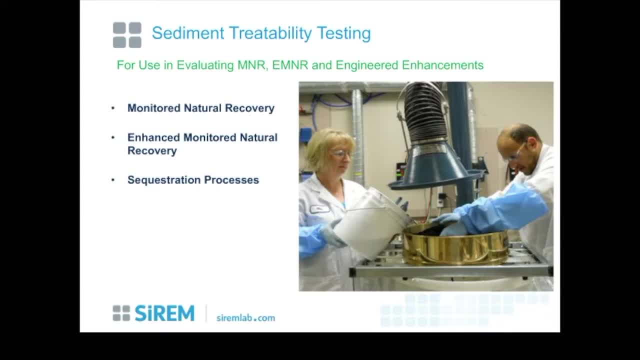 and institute chemical oxidation, where for sediment sites, they're looking at something called monitored natural recovery, which is natural attenuation. Enhanced monitored natural recovery is where you're adding or bio-stimulating a process to get degradation. Sequestration processes are where you're adding things. 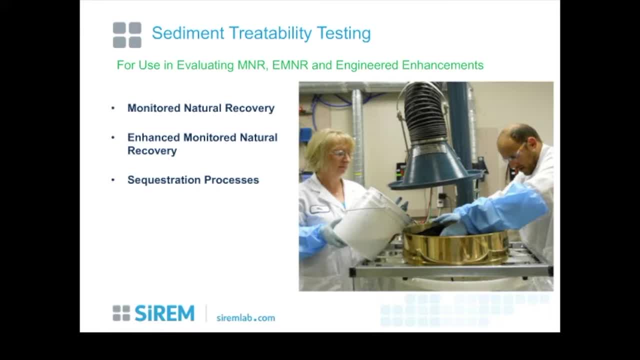 to perhaps cause uptake of contaminants into solid matrices where things are bound up and you don't get any further mobilization of contaminants. And again, these are often laboratory bench scale studies and we can use site materials. So the photograph here is buckets of site materials here being homogenized. 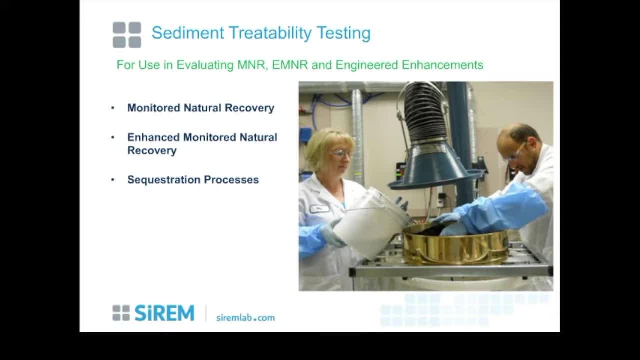 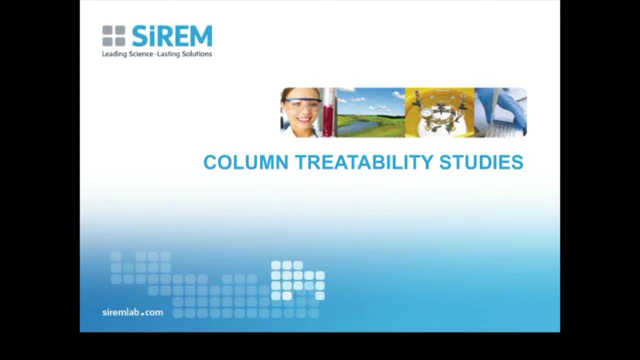 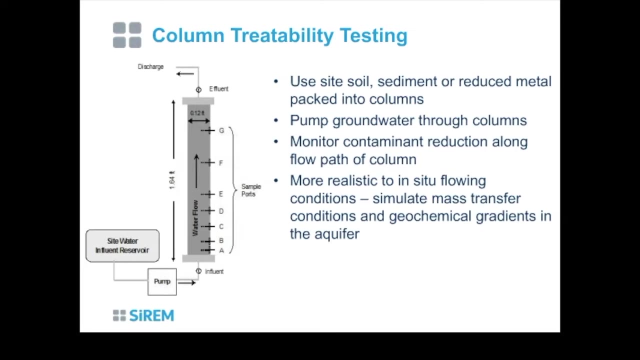 through a large sieve into a mixing tank before we made our microcosms. So now I'll touch on our column treatability studies. Our columns are upflow columns. We pack them either with site soil, sediment, reduced metal, whichever you want to evaluate. 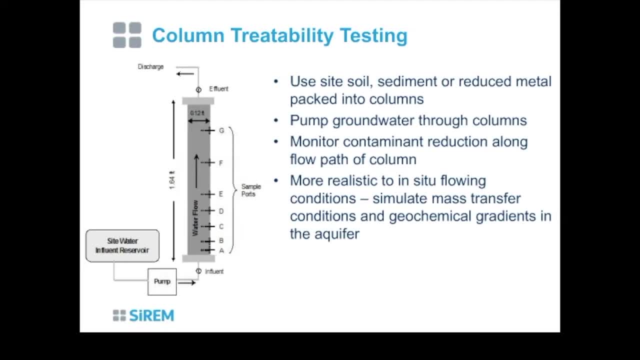 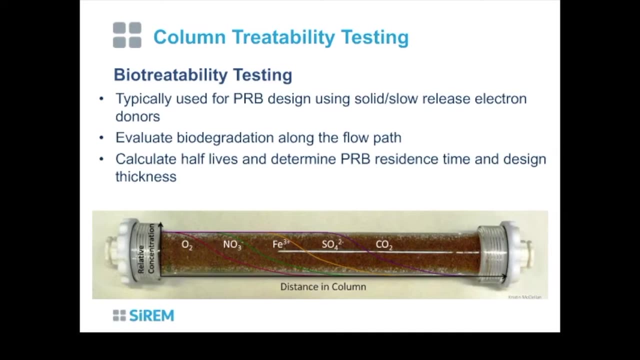 We do upflow pumping up through the columns and we monitor contaminant reduction along the flow of the column. It's more realistic to in-situ conditions and you can simulate mass transfer conditions and perhaps even observe some of the geochemical gradients that you might observe in the aquifer. 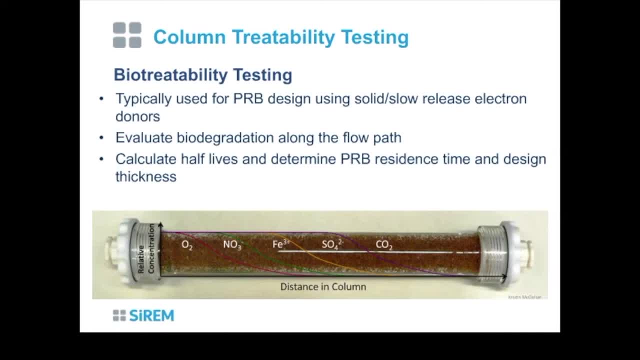 So for bio-treatability studies, these columns allow us to test for PRBs, so permeable reactive barrier designs, where you're looking at solid or slow-release electron donors And you can see the gradient of conditions where the front of your column study. 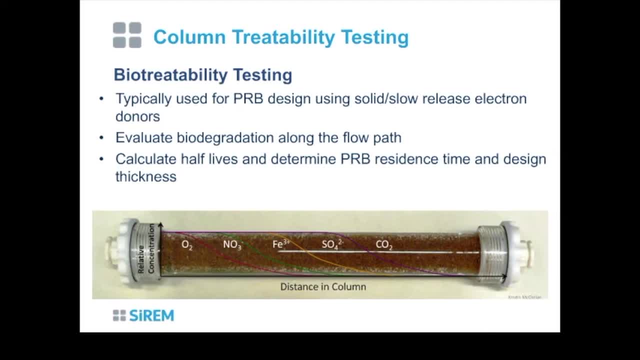 you might see reduction of any aerobic conditions or oxygen, then nitrate-reducing conditions, iron-reducing, sulfate and methanogenic conditions. ultimately, It allows you to evaluate biodegradation along the flow path, calculate some half-lives, look at resident time. 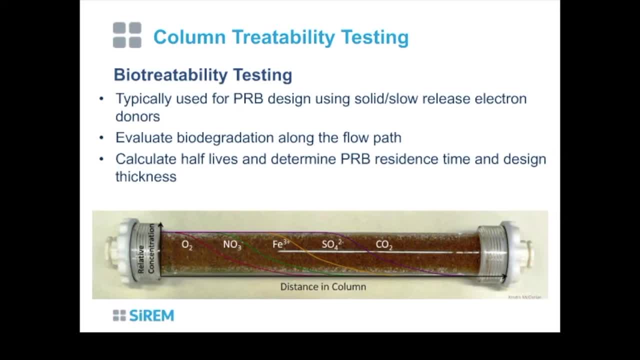 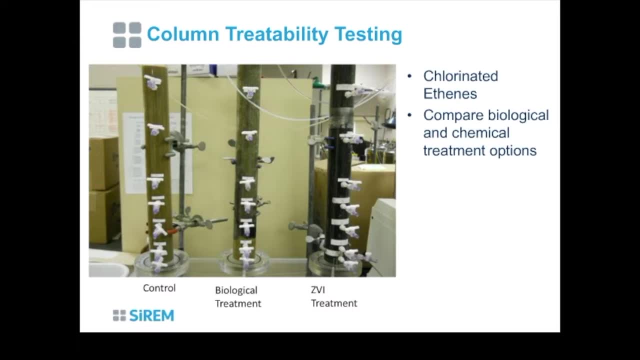 and design thickness, So it can be quite a valuable tool to providing design data. Here's some photographs of some actual columns set up in the laboratory. One thing I'd like to point out is the zero-valent iron is actually black, so we've got granular zero-valent iron packed into the column here. 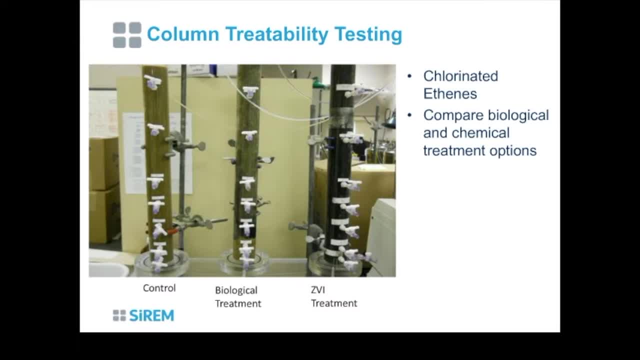 We have a control here where we're not adding any amendments at all. In the biological column here we've been adding electron donor And what we see here is we see once the reducing conditions were established. you can see the blackening of the column around this port right here that I'm circling. 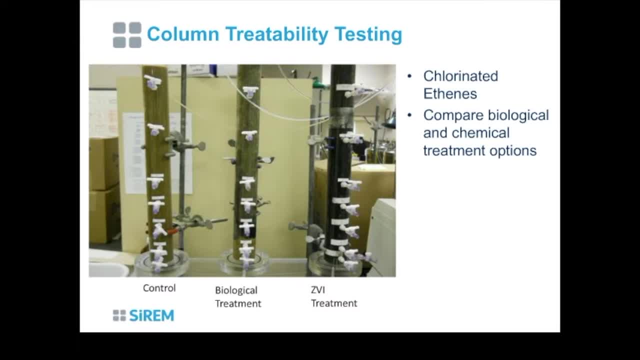 and that shows where we had establishment of reducing conditions for anaerobic bioremediation. We typically run 40 pore volumes. ZVI columns run typically six to eight weeks. Biological columns run six to 12 weeks. The processes are just different timeframes. 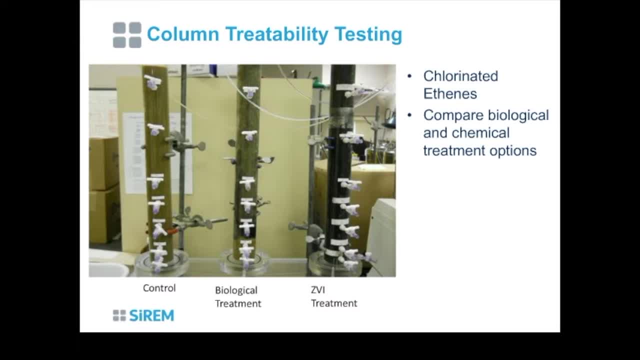 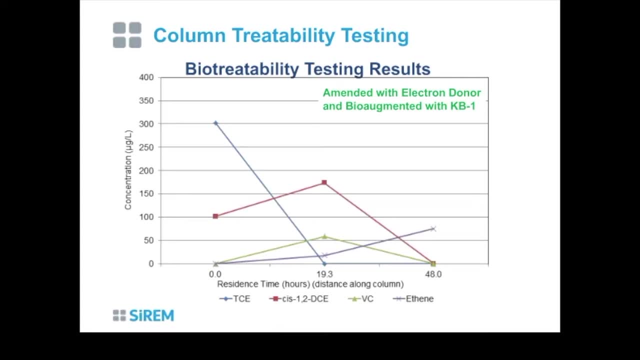 but they're very useful for doing evaluation in a flowing system. So I've got a little testing result here from a column study that we did in the laboratory. The resident time or the distance along the column is shown here and we only sampled at the influent, the middle port and the effluent port. 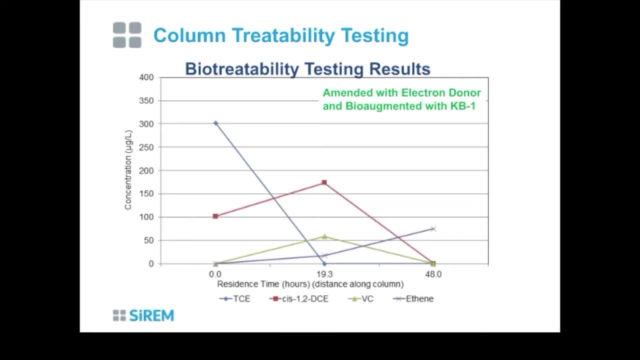 And we have concentration in micrograms per liter. looking at chlorinated ethene And you can see at the influent, we had cis-CCE and TCE in the influent groundwater. Midpoint of the column we saw some partial degradation. 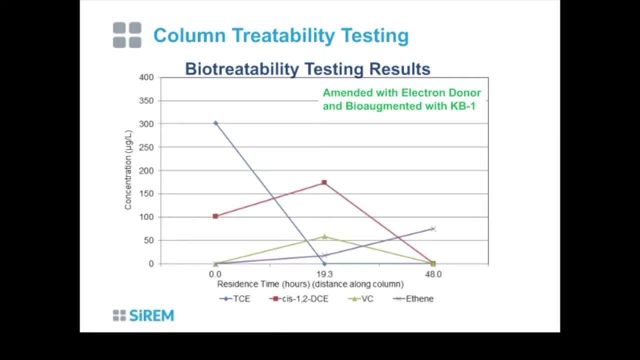 TCE is all gone, but we have cis-CCE and vinyl chloride still present, with only a little bit of ethene. And then we get at the end points, the only place where we only saw an end product breaking through, And it's very useful because this data can be then used to determine the minimum wall thickness. 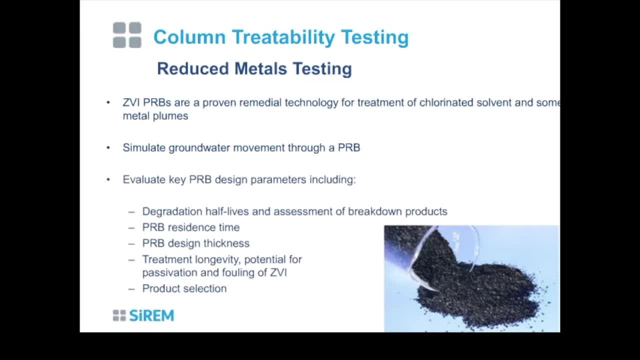 Reduced metal testing is being very widely used in column testing And the ZVI PRBs are well used in North America For treatment of chlorinated solvents and some metal plumes, And the design parameter data that you get allows you to understand degradation half-life. 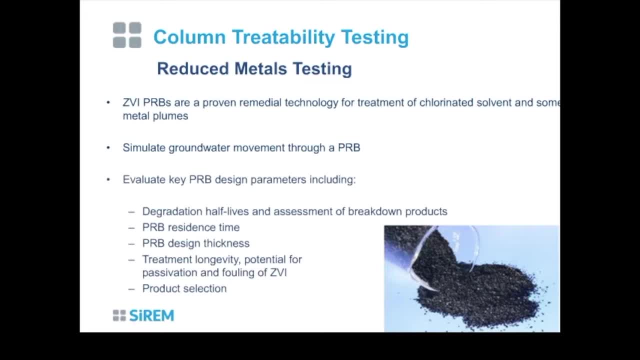 the resident time of your barrier, your design thickness, as well as looking at what might happen to your iron- Is there something about the geochemistry of the groundwater that will passivate or foul your ZVI? And also even product selection. so evaluating different types or grades of iron or different vendors of iron products. 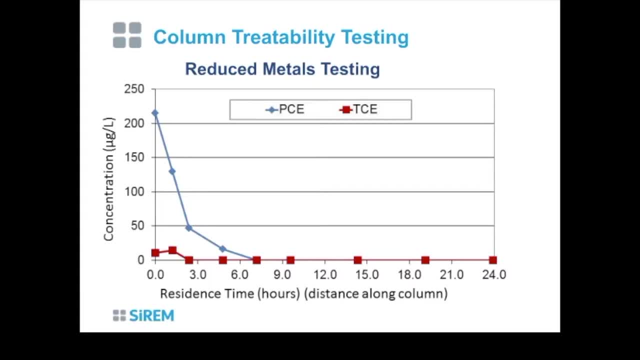 And so this is a snapshot at a discrete sampling event from a column study looking at zero-valent iron, where we see a resident time or distance along the column, And we have seven sample events over six to eight weeks. At each sampling event we get a snapshot, just like this. 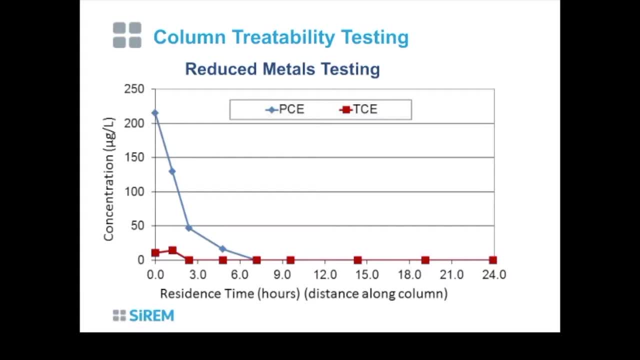 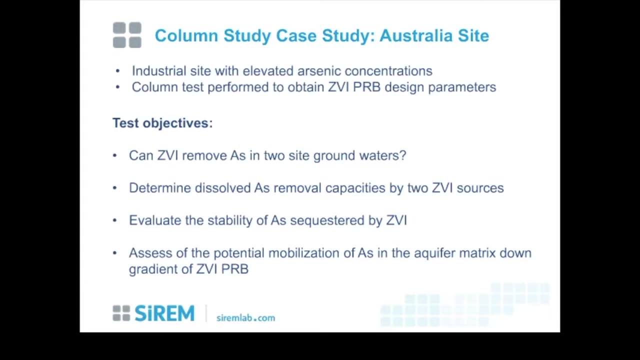 and we see different results. In this particular case we see the PCE and the TCE at the influence, which by about six hours resident time is completely degraded in this particular case. So I wanted to just do a case study for materials that we got from a site in Australia. 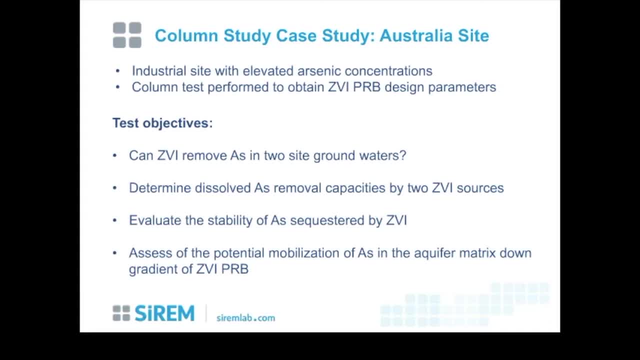 This is an industrial site that had elevated arsenic conditions and they were looking at understanding ZVI PRB design, And so they were very concerned about arsenic mobilization, and so they had a variety of different test objectives. So initially they said: 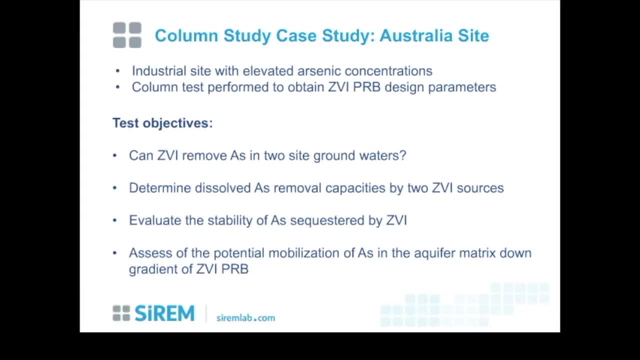 are we going to get treatment of the arsenic in two different site groundwaters? So they provided two different groundwaters. They also wanted to evaluate two different iron sources to see if either one had a better removal capacity, as well as look at the stability of arsenic sequestered by zero-valent iron. 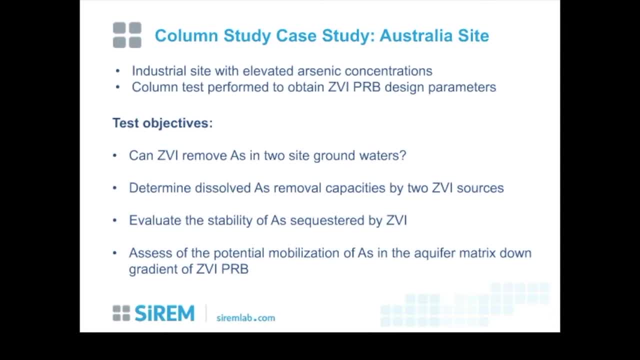 So the arsenic was sequestered into zero-valent iron and would it stably stay there or would there be conditions under which it would be released? So, looking at, because the receptor at the site was surface water, there was limitations as to where the barrier could be placed at the site. 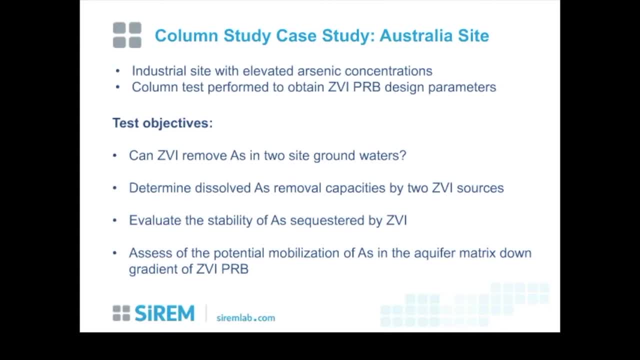 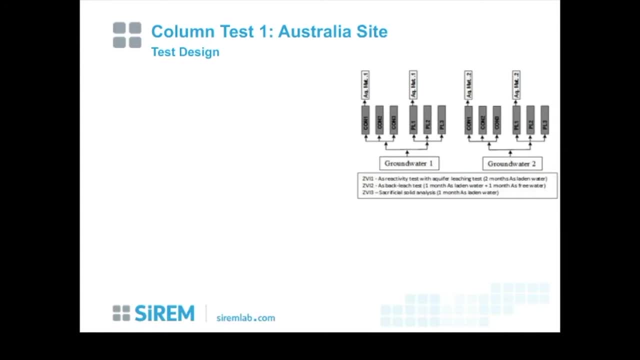 So they wanted to also look at the potential mobilization in the AXA matrix down gradient of any barrier that they were going to put in. So my picture did not come up. Hang on a second. There we go, So in this photograph here. 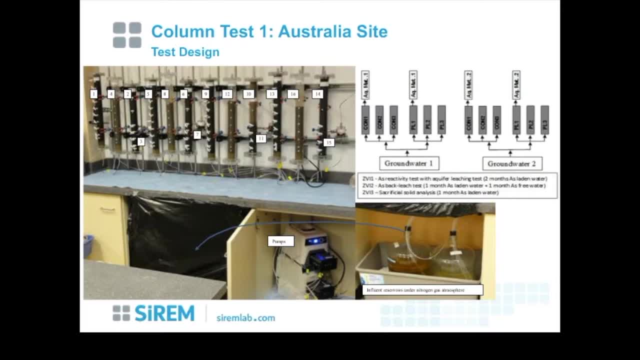 we have a picture of all the columns. Essentially I'm just going to walk through a set up and then there's four setups In the little schematic here on the right. it shows we had two different groundwaters. We had two different irons. 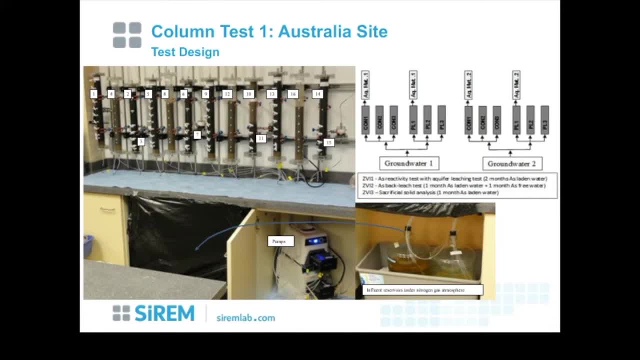 So there's groundwater one and groundwater two. Then there's the con iron and the PL iron. So each setup here is identical, just one different variable. So in this case, here we're looking at the con iron with groundwater two. This is the con iron with groundwater one. 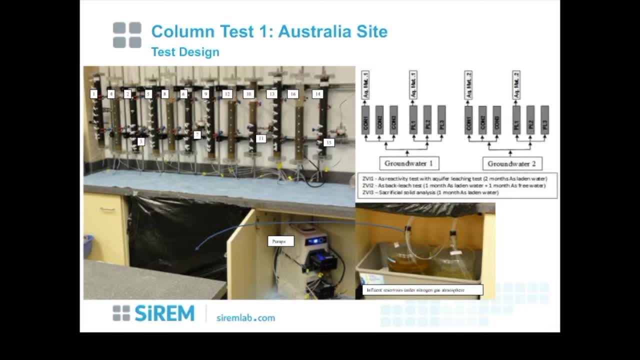 and then groundwater two Column one which is this one here was a ZVI to aquifer sequence and this allowed us to get information about arsenic removal capacity and if the arsenic would be mobilized down gradient because we took the effluent from the zero-valent iron column. 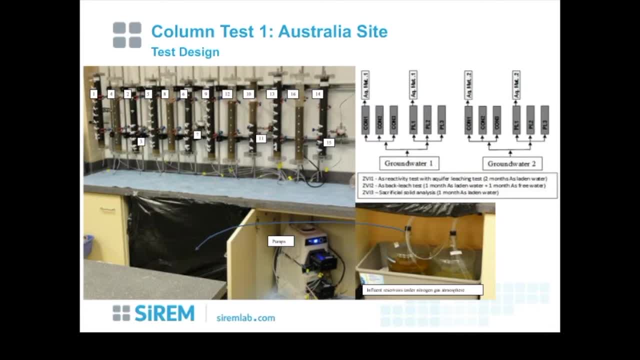 and put it through just an aquifer matrix column to see if the water coming off of that potential barrier would then strip any arsenic out of there. The column two was zero-valent iron, run for a month with arsenic impacted water And then flushed for an additional month. 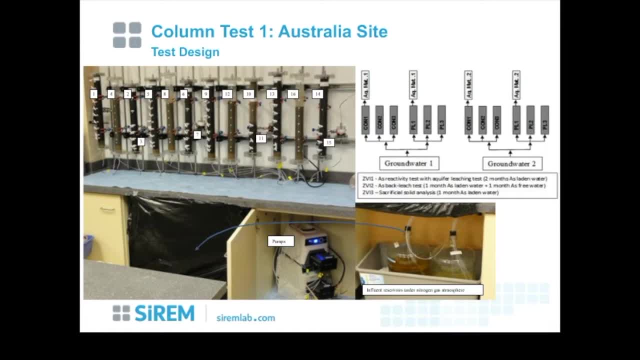 with arsenic-free water to determine if the arsenic would be back-leached from the zero-valent iron. And column three was essentially a replicate of column two, but used as a sacrificial sampling device so that we could sacrifice that sample for spectroscopy. 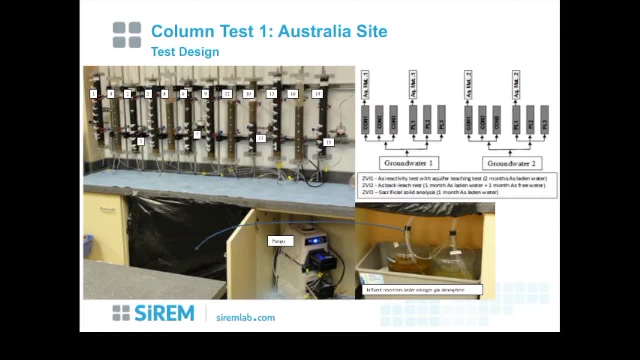 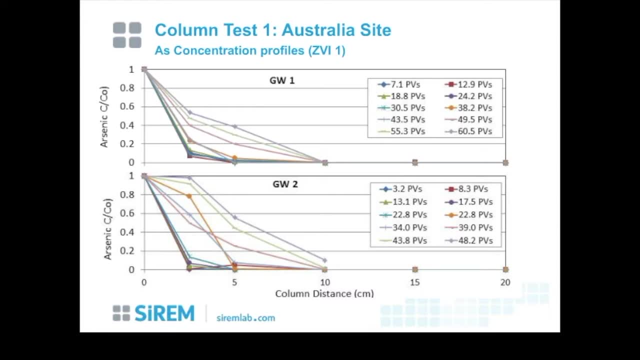 and some of the leaching experiments that needed to be done. So the results are shown for one iron type but two different groundwaters And this was the better performing iron. Just for the sake of time, I'm not going to show all the results. 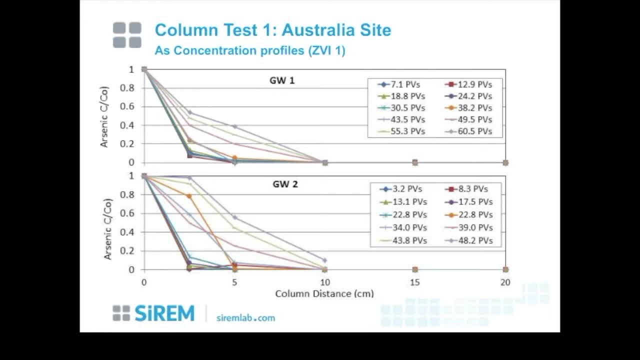 And what's shown is the C over C naught, so the concentration change over 10 profiles with increasing volume of water, And so these are essentially breakthrough curves And, as you see, the iron is getting used up or passivated, and so we see a progression of arsenic profiles. 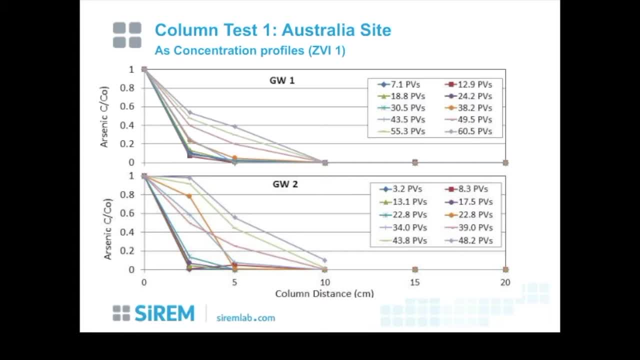 Arsenic five gets reduced to arsenic three and then complexes with iron and creates solid phases. So it creates passivation because it blocks the iron surfaces and doesn't allow it to be reactive any longer, And so you can see in groundwater one. 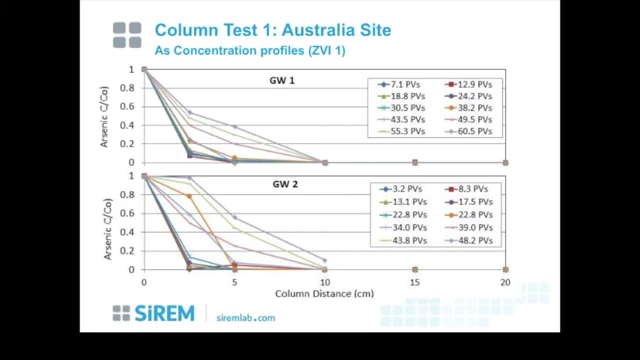 we did 60 pour volumes And you can see that at this port here that I'm pointing to, at 60 pour volumes we had breakthrough of the arsenic, whereas at seven pour volumes it was much less And you can see in groundwater. two: 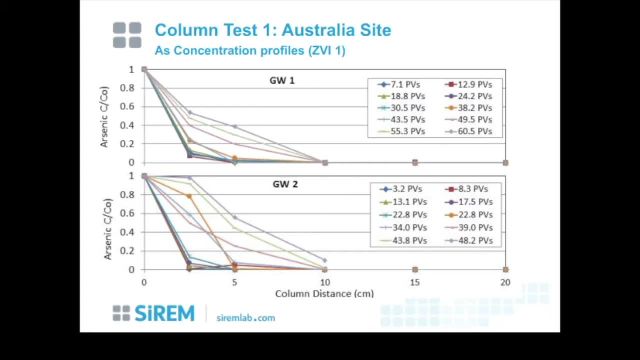 we had much better treatment at this first port and that, however, we did see breakthrough over time. Essentially in groundwater two, we had better removals but no reactivity with time and we had a lot less pour volumes in groundwater two. So we had some different results from each one of them. 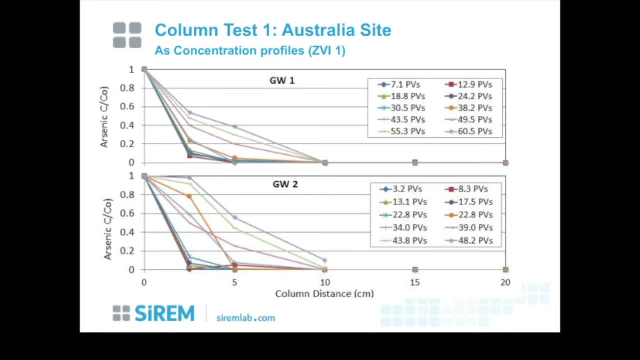 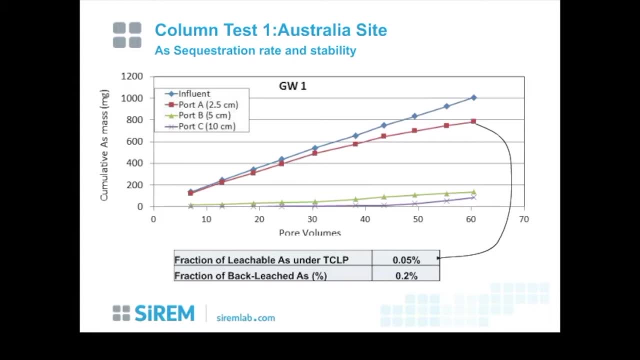 and they were very useful to the ultimate design of what they were going to use in the field. We also look at the cumulative mass of arsenic going through the column and what this plot just shows: that most of the arsenic was retained in the initial few centimeters of the column. 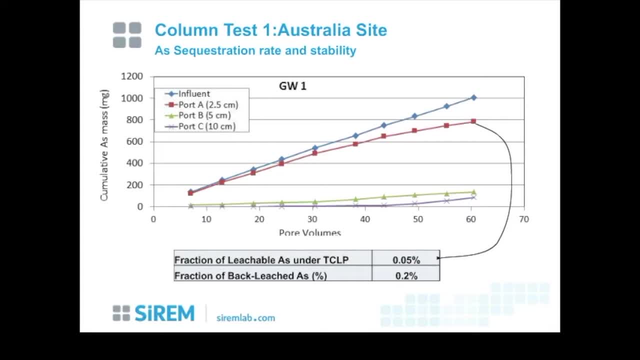 And so you can see that the influent is the blue arsenic concentration and port A, which is the first. after two and a half centimeters sampling port, the arsenic was there. And then what we did is we did leaching on the iron. 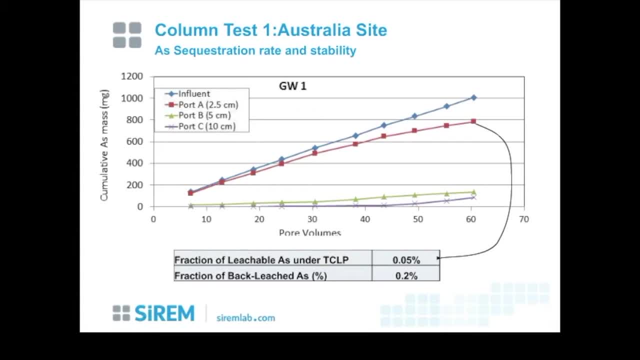 from that zone of the column and we indicated that the iron was strongly sequestered, And then, from the back leaching, we only determined that there was 0.2% of the arsenic that was leached. So essentially, the take-home message is that arsenic was strongly sequestered. 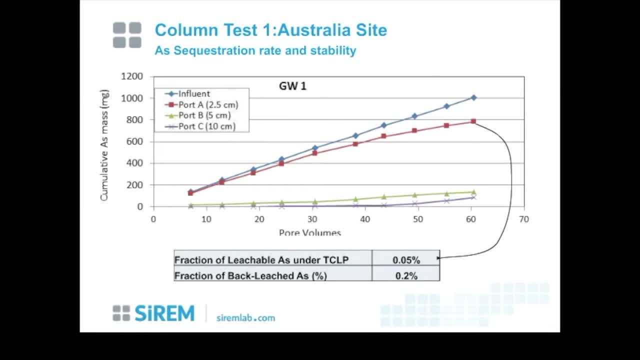 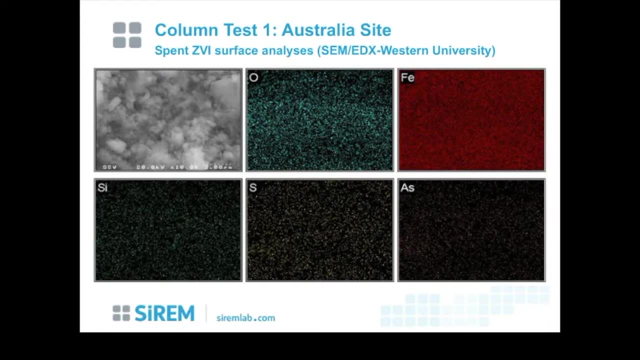 and not expected to be released from the spent iron. This is just a – I'm not going to go through all these results, but this technology was used, scanning electron microscopy with an energy-dispersive X-ray, and we used this to help understand. 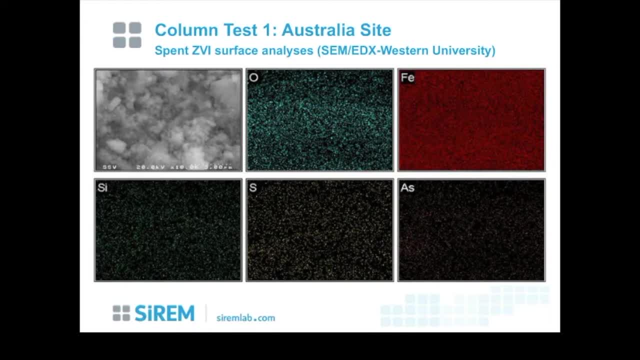 where the arsenic went and how stable it was. Essentially, it shows that the arsenic absorbed onto iron oxide surfaces and it was uniformly distributed, And so I'm not the expert in interpreting these ones. We use a local university, University of Western Ontario. 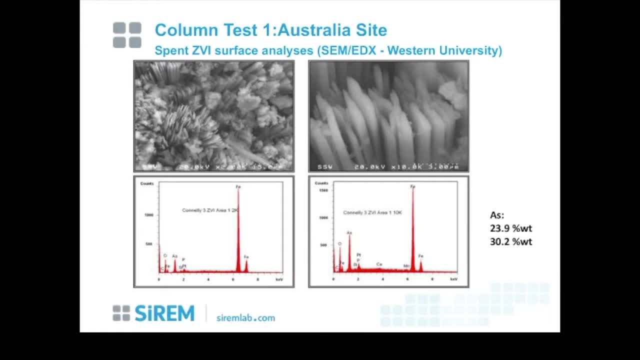 to help us interpret these results. And this next slide. here is the same technology, just a higher magnification: 2,000 X and then 1,000 X left and right, And it shows the actual crystals that developed on the iron grains. 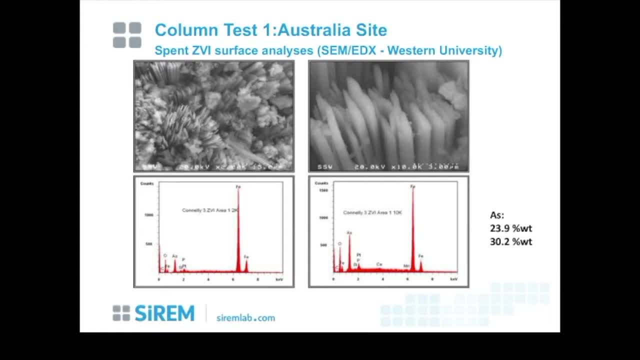 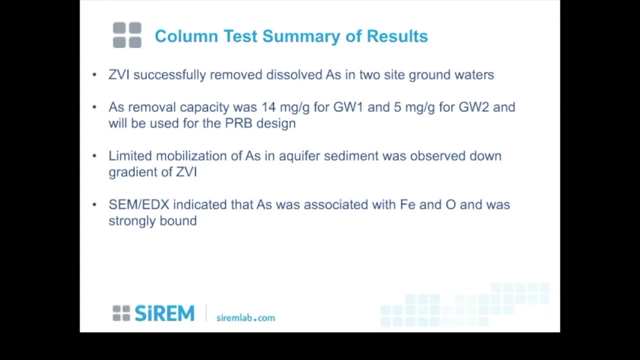 So all of this shows that the arsenic actually precipitated and created new secondary minerals with iron, which meant that it would be difficult for the arsenic to be removed with flushing. Again, just really good supportive information and data in understanding how the technology was going to work with the site groundwater. 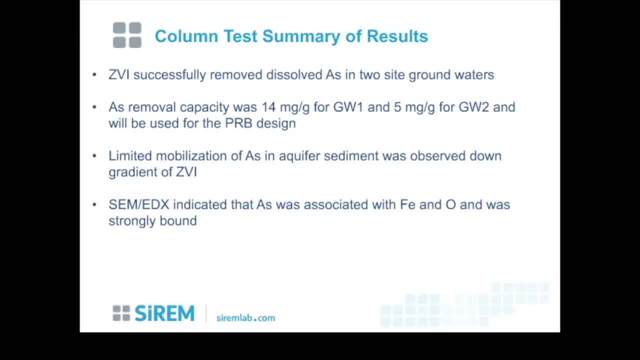 So again, we were able to successfully determine that ZVI removed dissolved arsenic- dissolved arsenic in the two site groundwaters. We were able to determine specific removal capacities that were used for the design. We were able to demonstrate that there was limited mobilization. 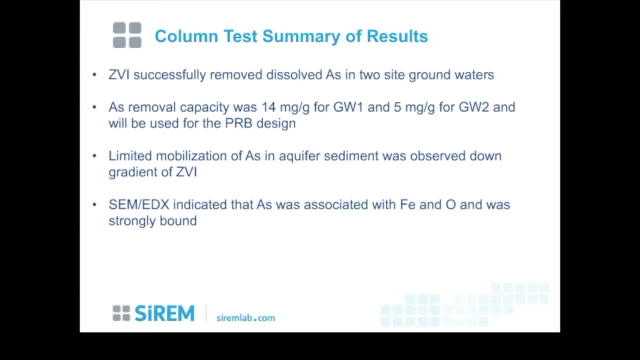 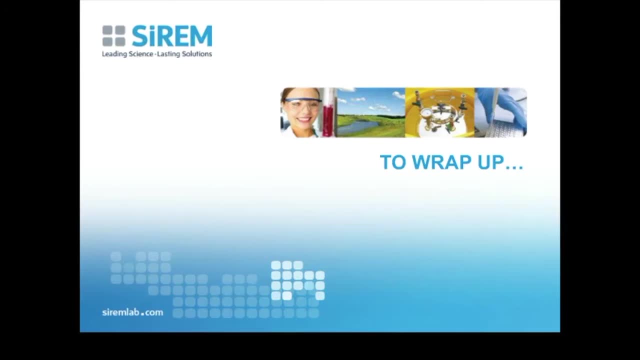 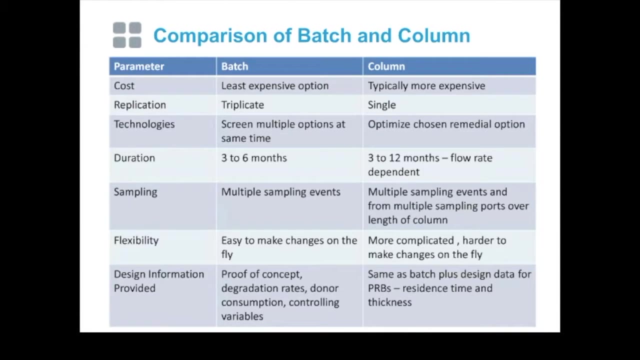 in the sediment down gradient of that And the scanning electron microscopy indicated where it was bound and that it was strongly bound. So I'm just going to start wrapping up now quickly so that we have some time for some questions. This table here is just a comparison of people wondering. 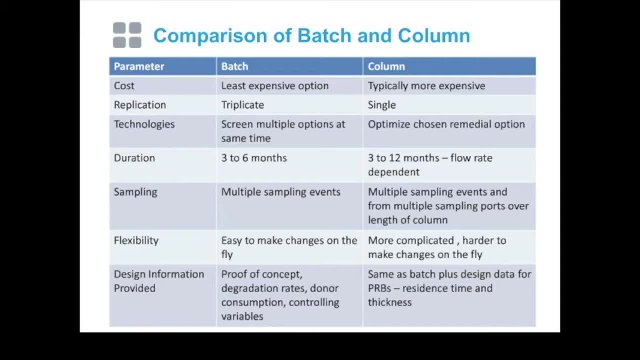 when would you do a batch versus column? And there's a lot of different factors And so batch studies are significantly less expensive than column studies. We typically do treatments in triplicate, whereas column studies because they're more time consuming and more expensive. 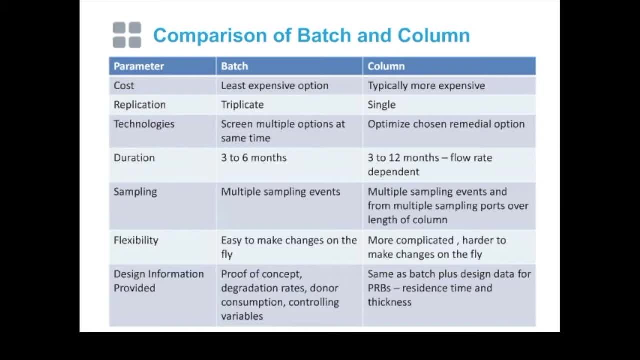 columns are typically done in single treatment. You can screen multiple options at the same time in a batch study and often column studies are used more of an optimization step. Batch studies are three to six months typically, but they often can run anywhere from four to 12 months also. 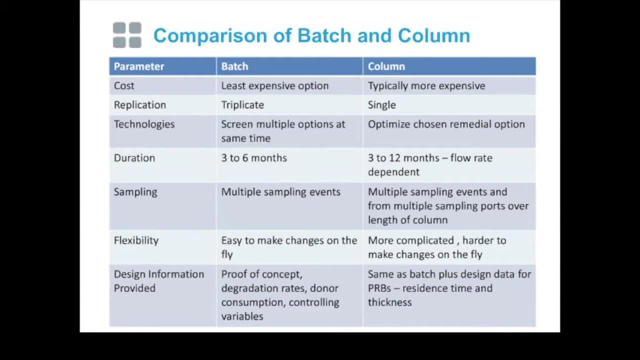 Column studies are flow rate dependent, so they can run anywhere from three to 12 months. Sampling events are multiple. for both of them, Again, there's differences in the flexibility of the types of studies, and the design information is significantly different as well. 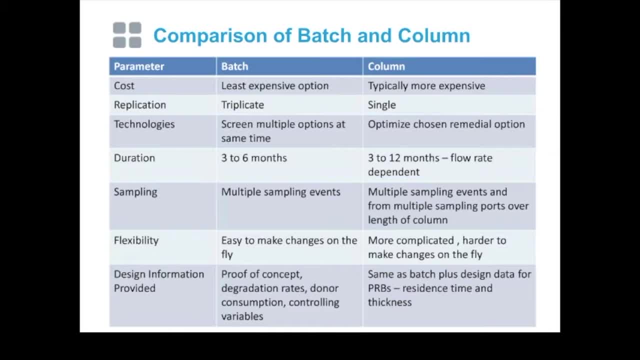 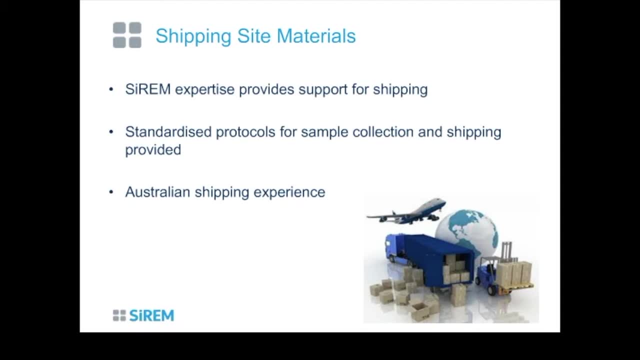 Batch studies are proof of concept. In column studies you do get more hard design data that can be used for design of reactive barriers. I wanted to touch on shipping materials to our laboratory in Canada. I've been doing treatability studies with materials from Australia. 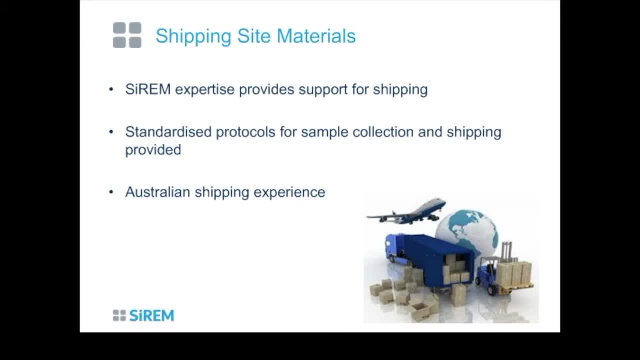 for a long time and it's relatively easy to ship to Canada. We have done it with success with a number of different sites And because environmental samples can be shipped as as limited quantity exemptions or as samples for destructive analysis, there typically is no regulatory issues with shipping materials. 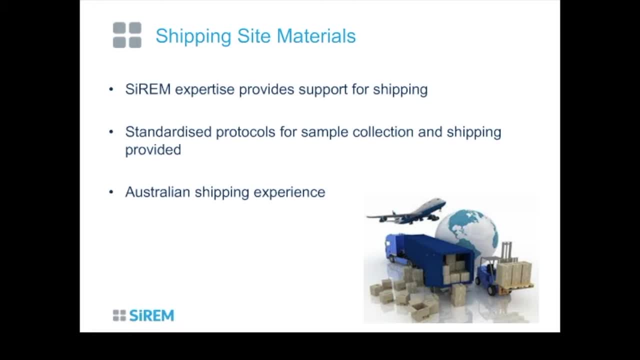 We can't call it soil. Agricultural soil would require a soil import permit, but typically most of the work that we do is sediment and geological material that's from the deeper subsurface, so it's not going to fall under the rules of the regulatory agencies. 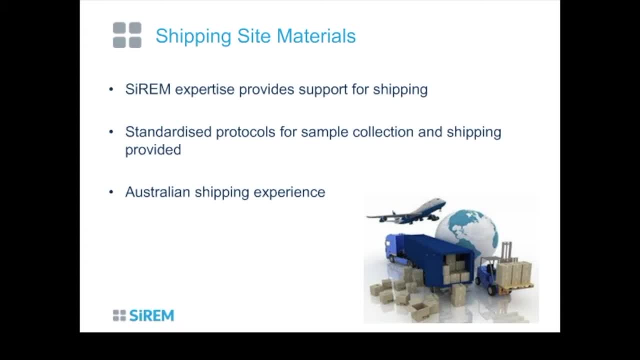 that are looking for soil pests and plant pathogens, which is typically why soil is regulated for its transport. But what we're going to transport is geological material, that's, you know, clay, silt, sands, gravels, and not things with plant roots and stuff like that in it. 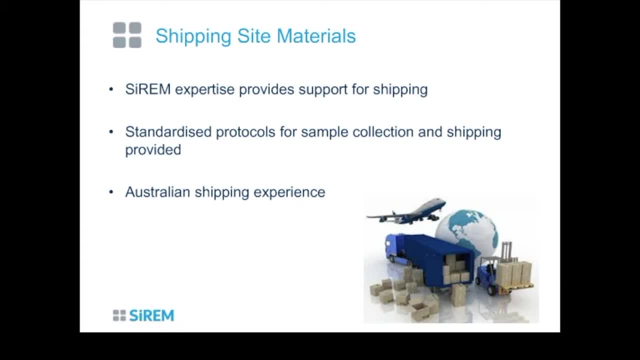 So we'll work with you to make sure you have the appropriate paperwork. We provide tracking of shipping and working out any. any hill holds that might occur, But with the right paperwork, shipments don't get held. I think that the point about packing your coolers 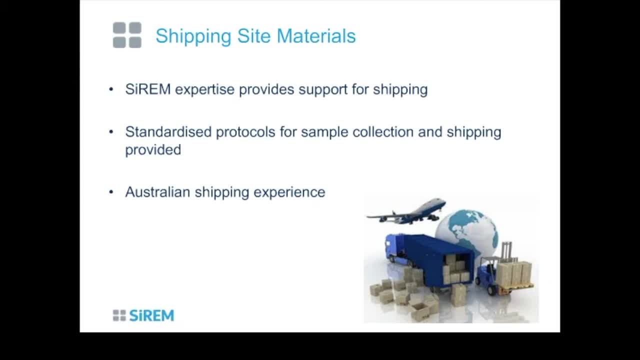 so they're not too heavy is very important. Often it's the weight that determines the cost, not necessarily the dimensions of the esky or the cooler that you're shipping, And so we've got standardized protocols that we provide for both sample collection and for shipping. 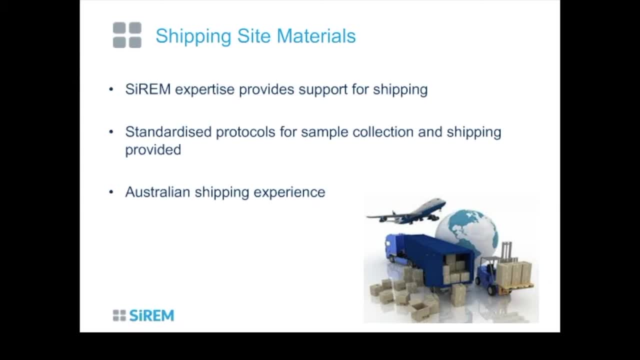 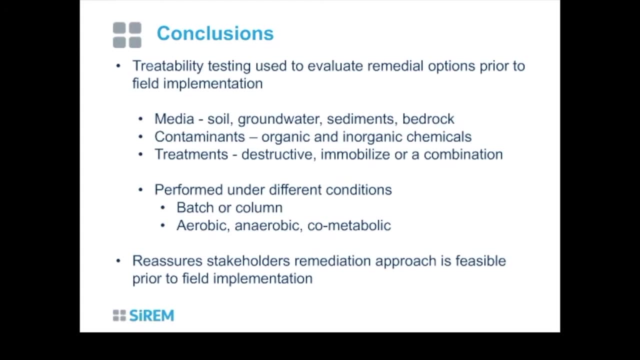 and we're always available, electronically or on the phone, to provide technical support and advice for shipping materials to us. So just wrapping up, finally, we have the resources to perform studies that allow us to fully understand some of your most challenging problems at sites and help you deliver solutions to complex problems. 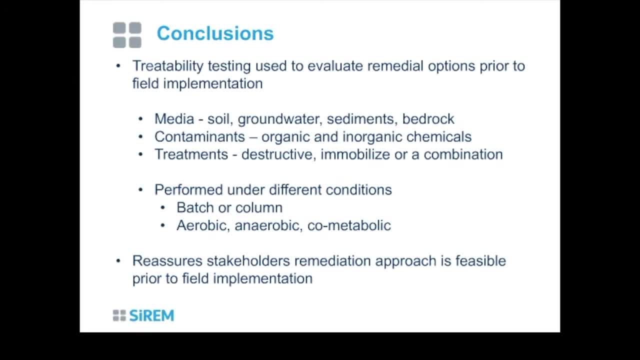 These studies can be performed for a variety of contaminants in many different media under many different conditions, And so we really are had a lot of success with treatability studies, and some of our best customers are repeat customers Once you get a good treatability study done. 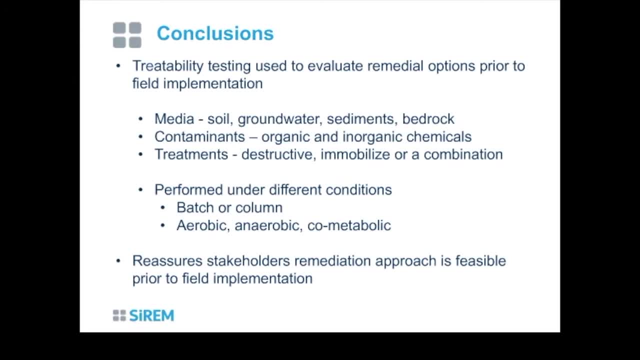 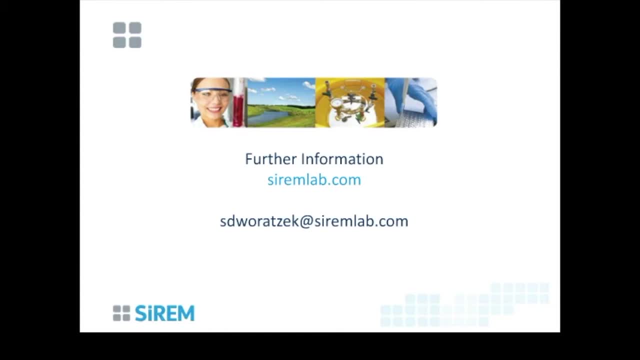 it's. they keep on coming back for more. We really enjoy good relationships with our customers in doing treatability studies And with that I will let Lang broker any questions that might pop up. Thank you for your time. Okay, Thank you, Sandra. 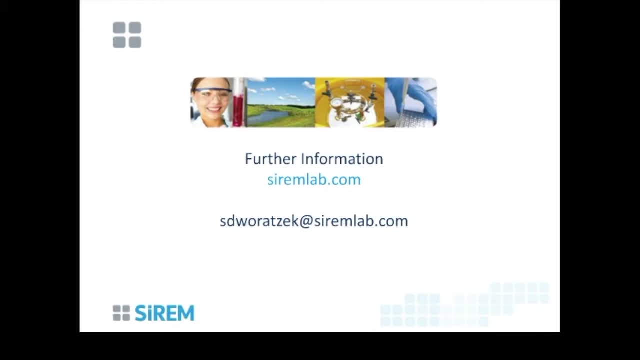 Very interesting presentation. Just before we march into questions, I'll just remind people that we will make available a copy of the webinar recording. It'll be a web and audio copy that will be available for download. I'll let you know when that's available. 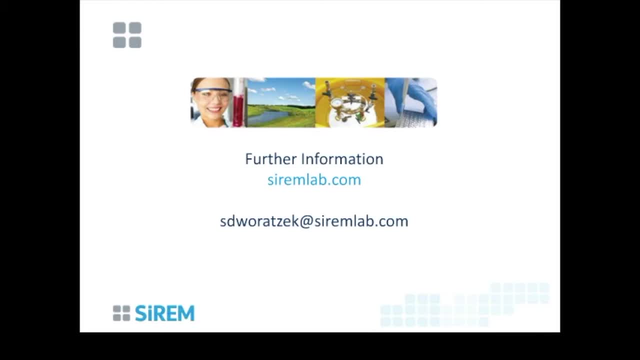 PDF copies of the slides will also be available if you want to be able to review those separately, But we would gladly take any questions from the group. If you want to ask them using audio. just click the arrow next to your name on the left of the screen and unmute yourself. 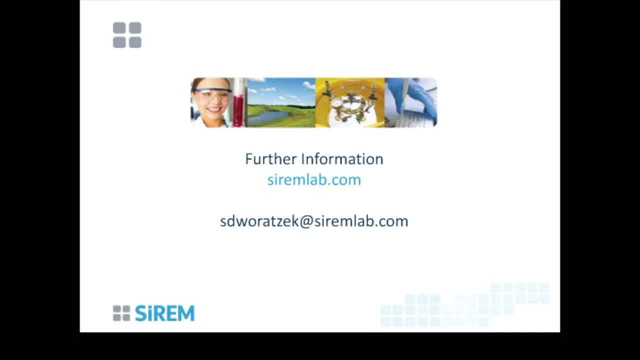 Otherwise, give the Q&A button at the top to go and we'll answer any questions from the group. I might ask one in the interim: Sandra: how many Australian sites do you reckon we've performed treatability studies for That's a good question. 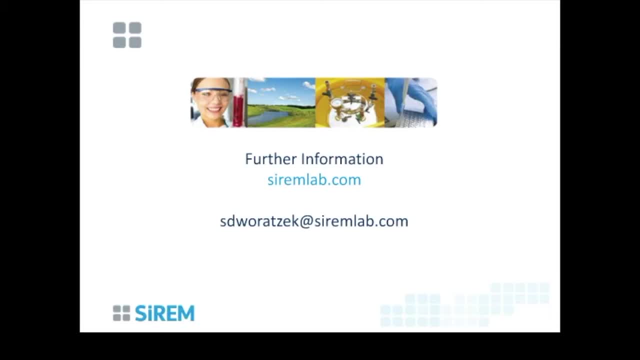 At least a dozen or more. I actually haven't got a tally for all of Australia, but I know that one of the first ones I did back in oh gosh 2000,, before Serum was actually officially Serum was for one of the sites in Australia. 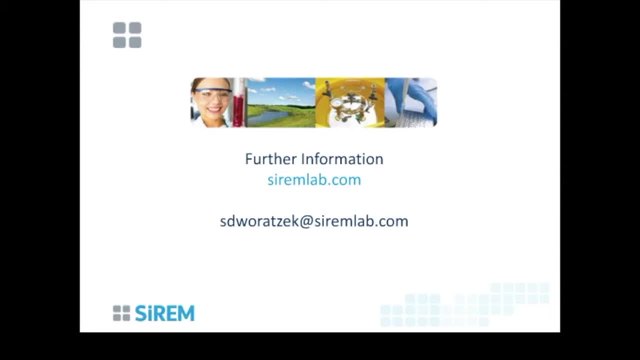 So we were looking at 1,2-DCA or EDC degradation. Are there any questions from the rest of the group out there? Happy to take anything now. happy to take anything via email afterwards as well. I'll follow up with an email to all the attendees. 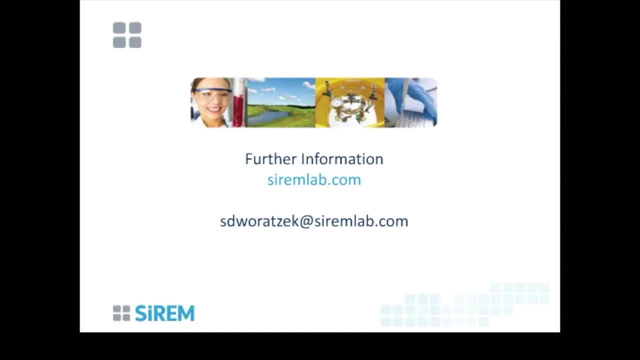 that has our contact details. so we're more than happy to take questions afterwards if you prefer not to ask now, But please do feel free if you've got any burning questions right now. Okay, Prashant, I see there's a question coming through in a moment. 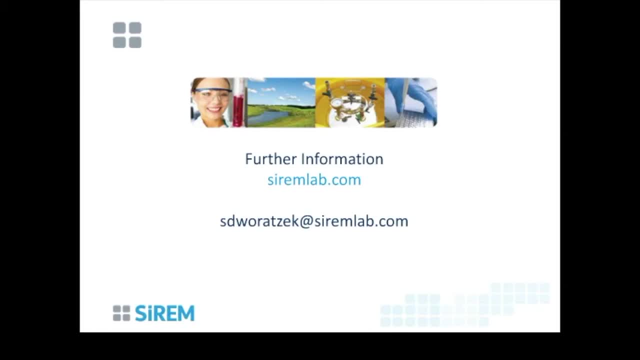 Probably being formulaic. so as soon as that comes through, we'll address that one. Okay, Sandra, can you see that question on your screen? No, I can't. Okay, let me read it out. It says: replicates are important in any treatability study. 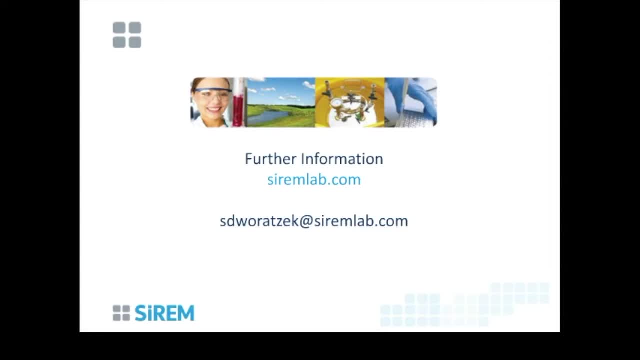 given. the results are going to be used to conduct a pilot trial or even a full-scale trial. Also, soil is a heterogeneous matrix. Why is it that you recommend a single replicate for column study? For column studies, it's cost, typically. what drives it? 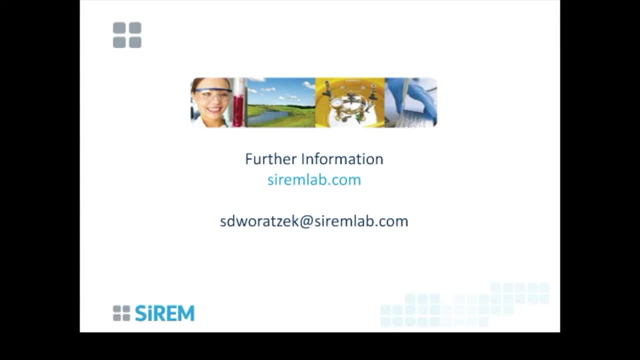 A triplicate column study is much more expensive, whereas triplicate batch studies are. it's not as expensive, And so, for column studies, if someone wants to do it in triplicate, we'll certainly do it, but I think it's the cost that would drive the decision. 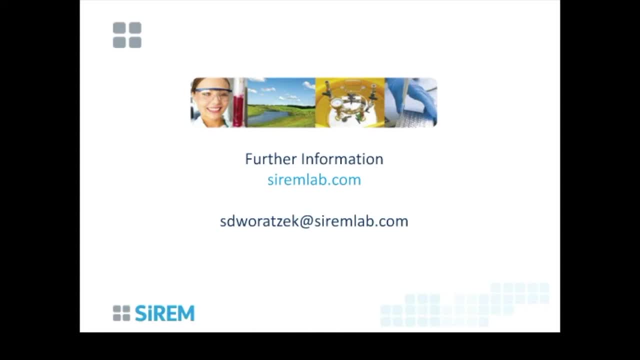 You certainly can use a much larger sample size in a column study. You'll be using upwards of perhaps a couple of liters of soil in a column study, so you do have a larger sample size of the soil, whereas in batch studies the microcosms often only have 75 to 100 grams of soil. 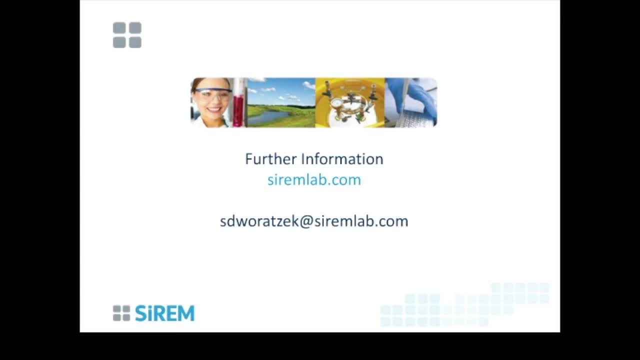 in those ones. Okay, there's another question that came through the Q&A- It looks like from Simon Mills. It says: Hi, Sandra, have you found persulfate with base activation is effective for petroleum hydrocarbon remediation in soils or sediments? 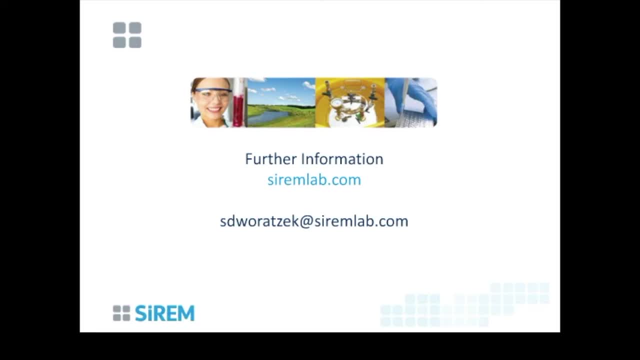 We've done some trials in our lab over two to seven days and the process seems very slow compared to the expectations of some consultants. Do you have any thoughts on that one, Sandra, Yeah, Yes, we've found similar results, but you don't get as. 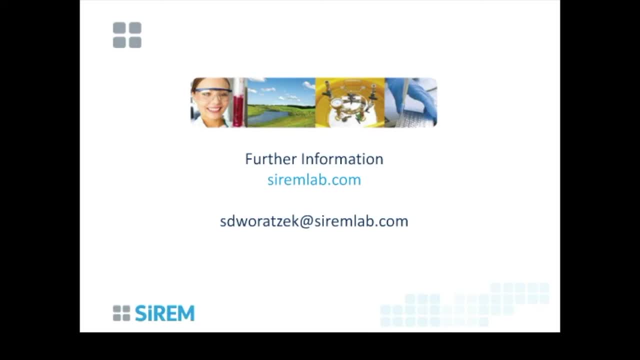 depending on the petroleum hydrocarbon mixture, base activation may not be strong enough. Often the trials, the challenges are the base activation. So we've done a lot of research on the base activation itself. Often we'll do in our oxidant studies. 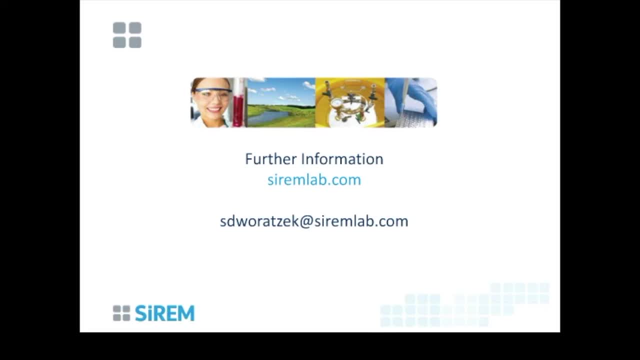 an evaluation of how much hydroxide is required to keep the pH above 10.5 or even above 11 to keep the persulfate activated. And we certainly see, depending on which petroleum hydrocarbon, different effectiveness And sometimes it works and sometimes it doesn't.